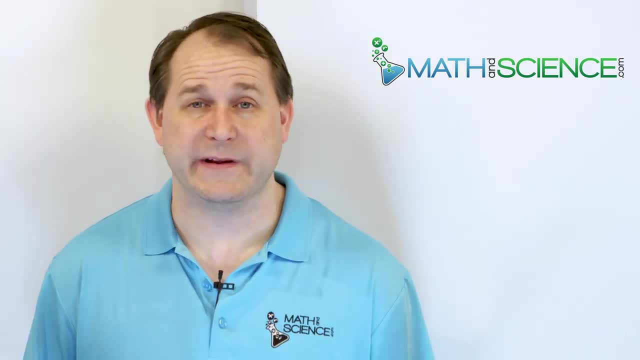 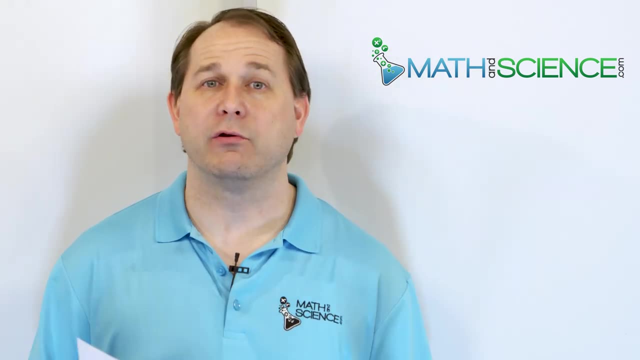 logarithmic equations and simplify expressions, but I never proved them to you And I want to take a minute to prove them to you because I don't like telling you: hey, this is true, trust me, In general, I don't like to. You probably could skip this section if you want to. 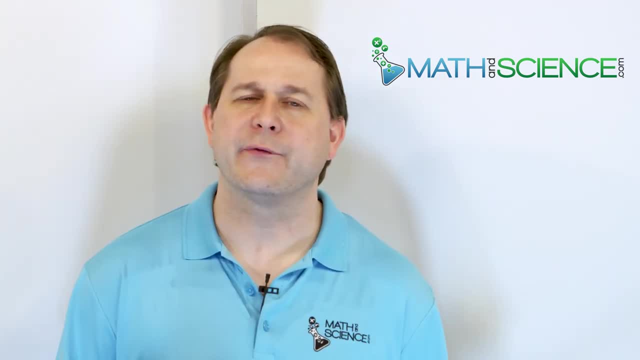 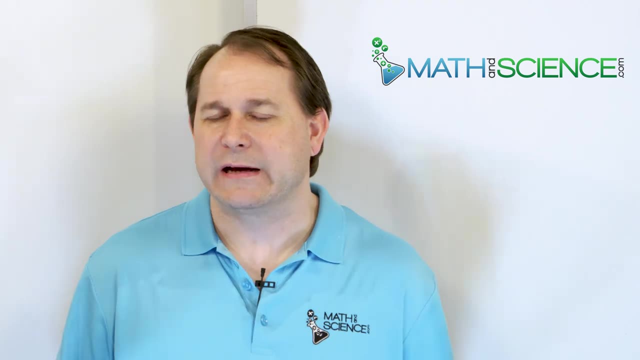 but I think it's probably a good idea that you watch it, just so you can know where they come from And also because it's a good exercise in working and manipulating logarithms. So you get your skills, kind of like, you get your skills sharpened as well. So at the end of this, 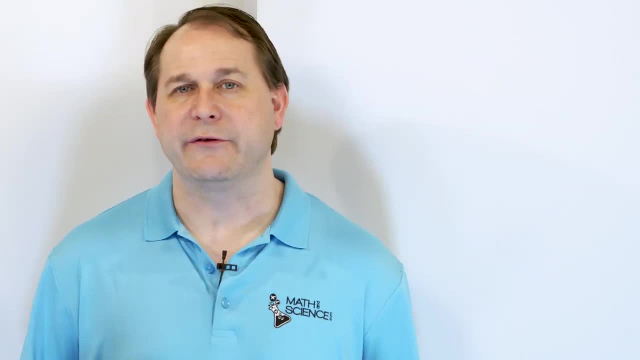 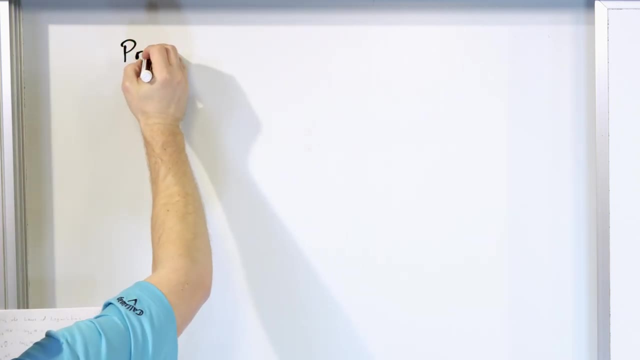 I really like you to prove them all yourself, Even after you've seen me do it. there's a lot of use in that. So we're going to prove three laws of logarithms here. The first one we're going to prove is the following: We're going to prove the one that we use all the time. Well, 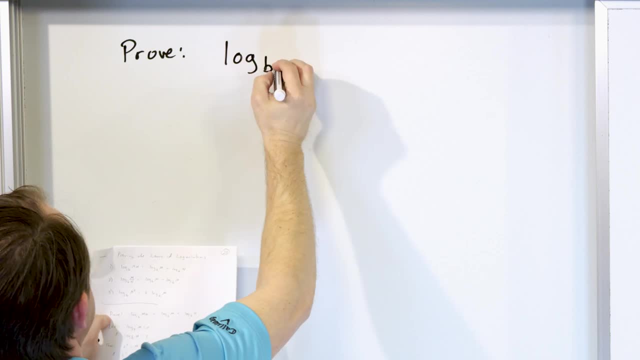 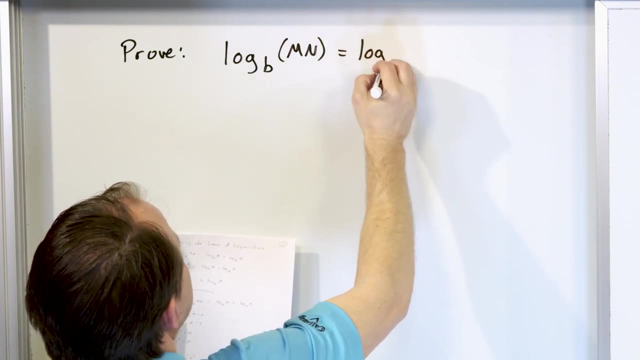 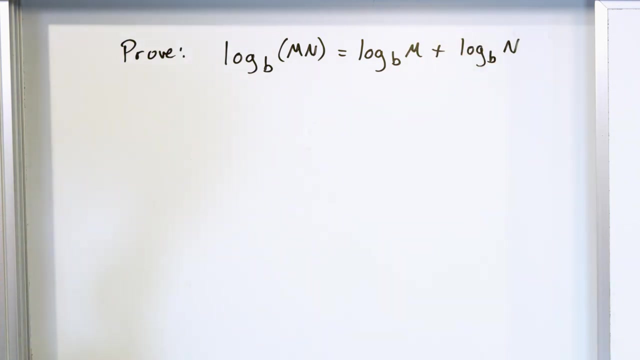 we use all of these, but this one we probably use the most. We use log base b of the product m times n And we now know, because we've been using this so much, that that's the same thing as log base b of m plus log base b of n. So why is it that when you 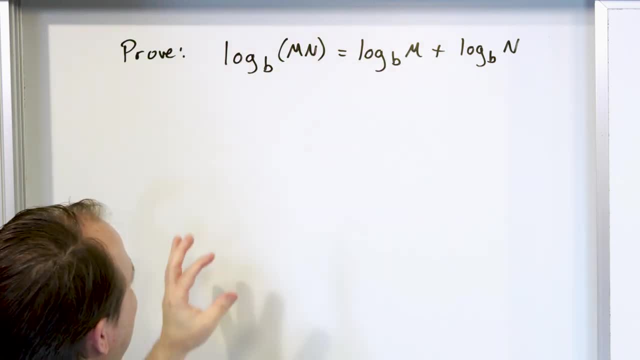 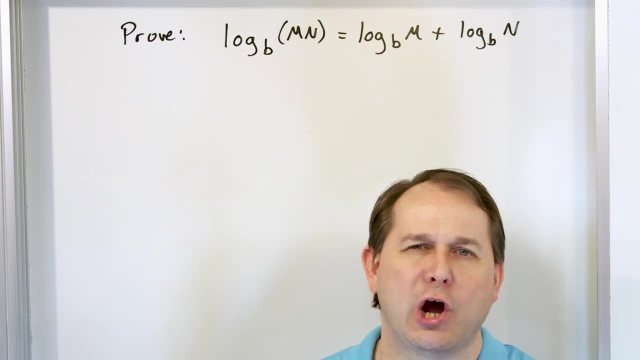 have two things multiplied in a logarithm operating on it, why does that become the addition of two logarithms? It's almost like multiplication. when you're dealing with logarithms You take the log of multiplication. it kind of gets transformed into addition of logarithms. So 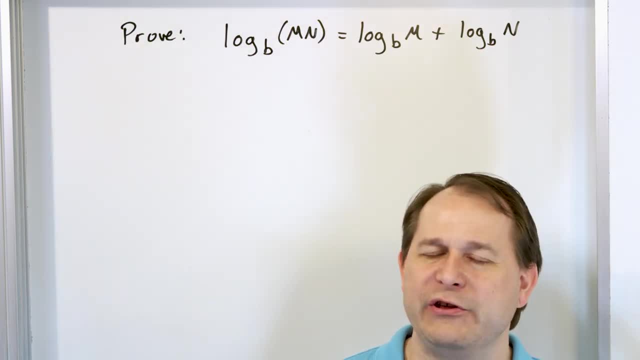 multiplication operation becomes addition, which is very useful for more advanced math. when we're trying to simplify things, Sometimes multiplying things gets tricky and dicey. You can change it to addition if you just take the logarithm of the thing. So we're trying to prove this thing here. 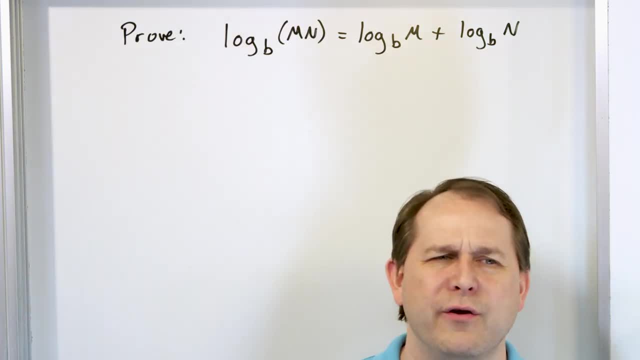 Also one more thing I'm going to say. probably in the beginning you might say, oh, that proof was neat, but I never would have thought of that. That's okay. None of us think of this stuff to begin with, right, You have to see it, right? As long as you understand what I'm. 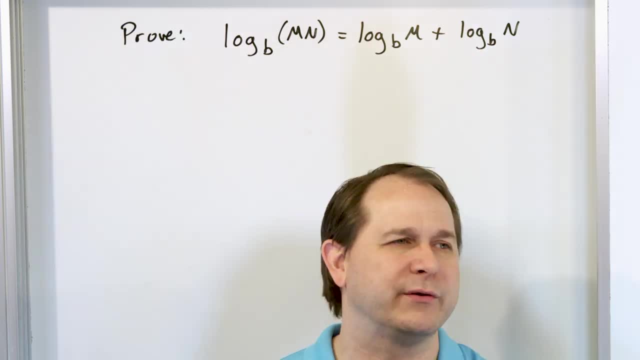 doing. that's all I care about. I don't expect you to know how to prove this. I don't expect you to feel you know- like you should already know- how to do this. I just want you to follow it, That's. 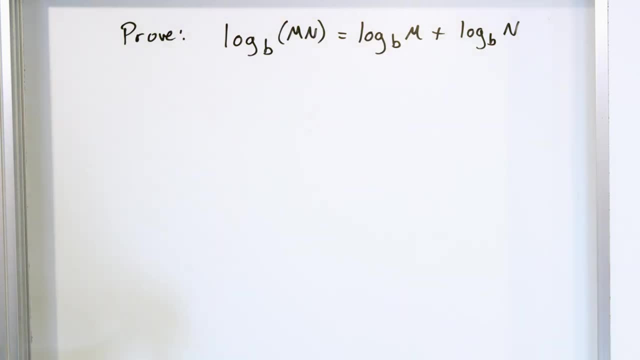 all I want you to do so that you can sharpen your skills. All right, So in order to do this, we know we want to add these guys together. So, to make things easier, let's let the following things be true: Let's let some new variable x equal the log base b of m, And let's let a new 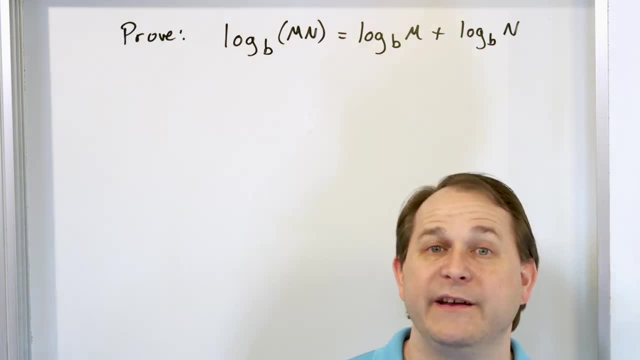 logarithms. So the multiplication of two logarithms becomes the addition of two logarithms. multiplication operation becomes addition, which is very useful for more advanced math when we're trying to simplify things. Sometimes multiplying things gets tricky and dicey. You can change it. 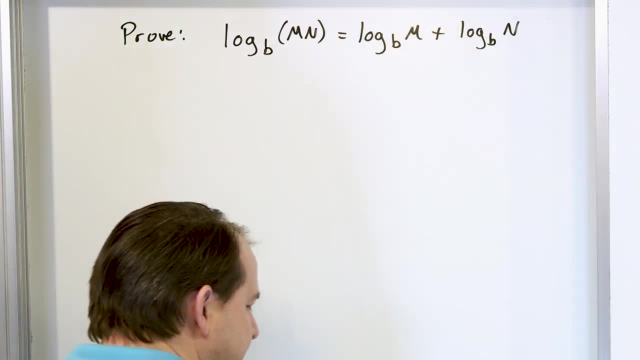 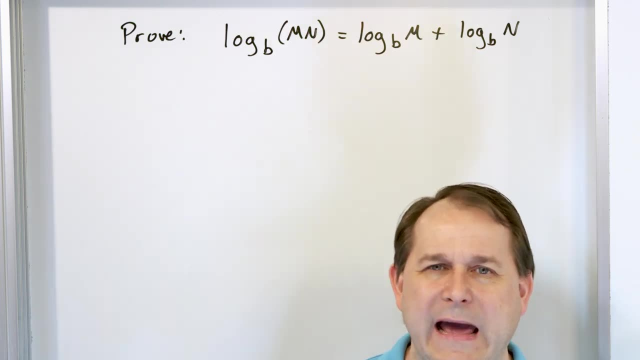 to addition, if you just take the logarithm of the thing. So we're trying to prove this thing here. Also. one more thing I'm going to say. probably in the beginning you might say, oh, that proof was neat, but I never would have thought of that. That's okay, None of us think. 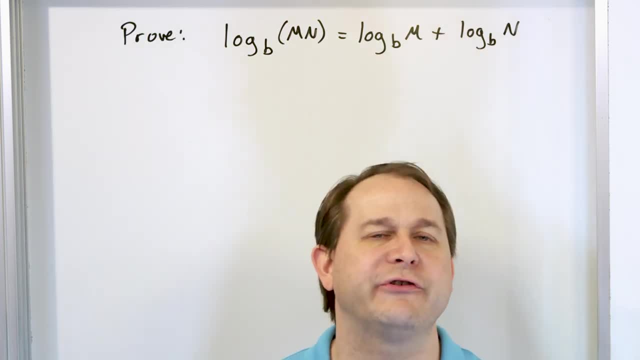 of this stuff to begin with. right, You have to see it right. As long as you understand what I'm doing, that's all I care about. I don't expect you to know how to prove this. I don't expect you. 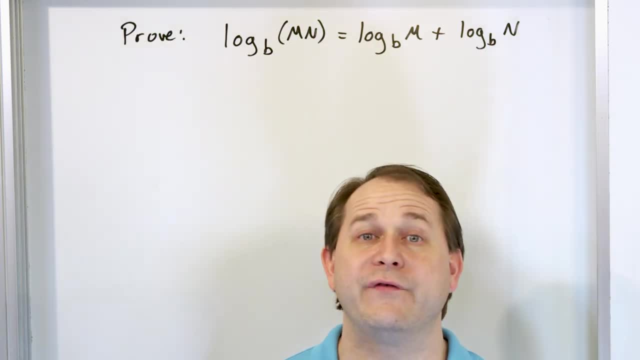 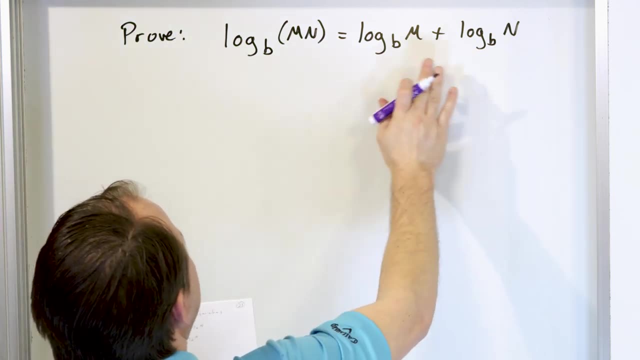 to feel like you should already know how to do this. I just want you to follow it. That's all I want you to do, so that you can sharpen your skills. All right, So, in order to do this, we know we want to add these guys together. So, to make things easier, let's let the following 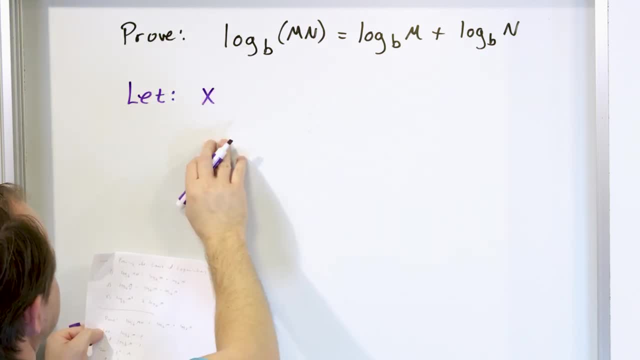 things be true. Let's let some new variable x equal the log base b of m, And let's let a new variable y be log base b of m. And let's let a new variable y be log base b of m, And let's let a. 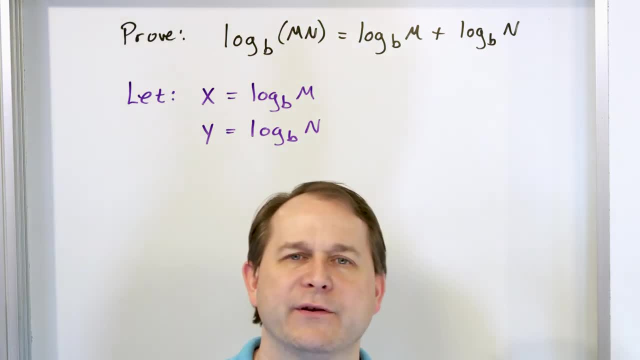 new variable y be log base b of n. You might say: why am I introducing new variables? Well, that happens all the time in proofs. The proof is like it's like a blank canvas for you to paint on. You can paint anything, I can paint what I want. I can paint Jupiter or Saturn, I can paint. 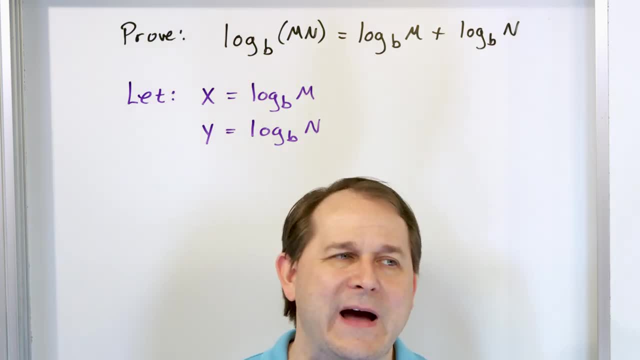 cows or chickens. It's whatever I want to do In the proof. I can do what I want as long as it's mathematically legal. So I'm just going to let the variable x equal to this and this equal to this. 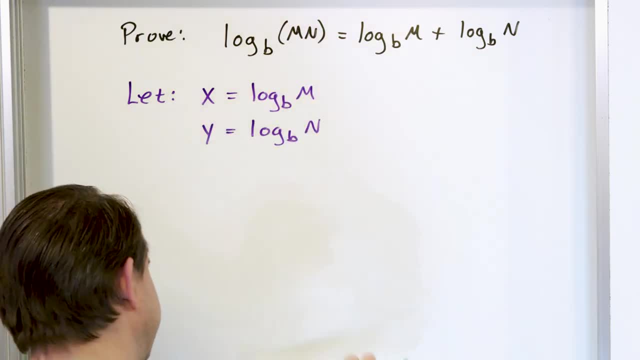 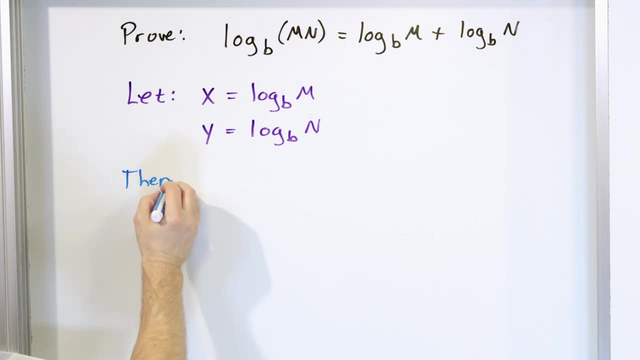 That's fine. The rest of it. I'm going to try to logically connect the dots and make this thing be true. Okay, But if I let these things true, then the following things are true, Because this is a logarithm. then I then know: because of this first line, b to the power of x is equal to m. b to the power. 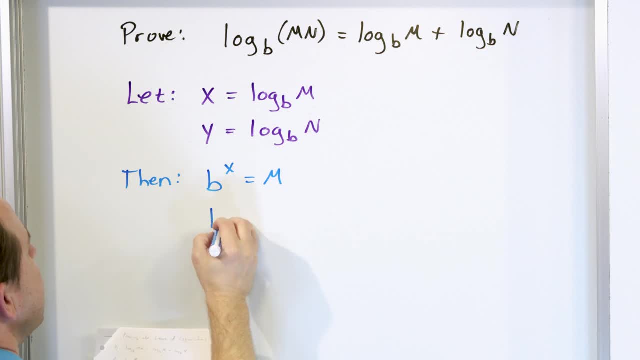 of x is m. That's a definition of a logarithm. And also b to the power of y is equal to n. So because of what I let these variables equal. then these variables are equal. You might say: this is not at all looking like that. That's fine, That's what I said. 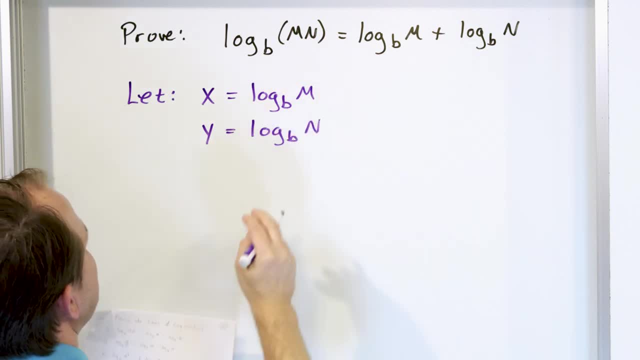 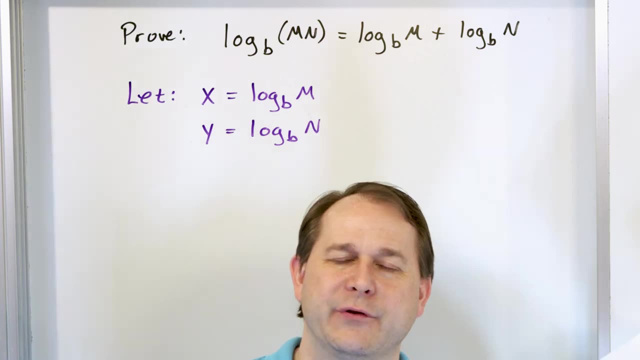 variable y be log base b of n. You might say: why am I introducing new variables? Well, that happens, time and proofs. The proof is like it's like a blank canvas for you to paint on. You can paint anything. I can paint what I want. I can paint Jupiter or Saturn. I can paint cows or chickens. 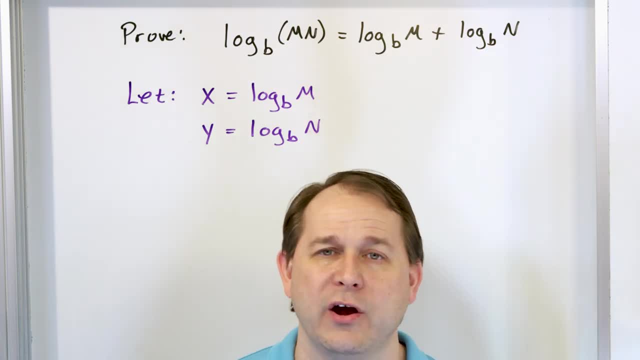 It's whatever I want to do In the proof. I can do what I want as long as it's mathematically legal. So I'm just going to let the variable x equal to this and this equal to this. That's fine. 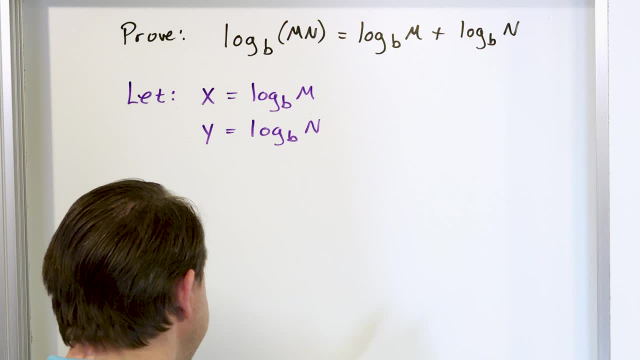 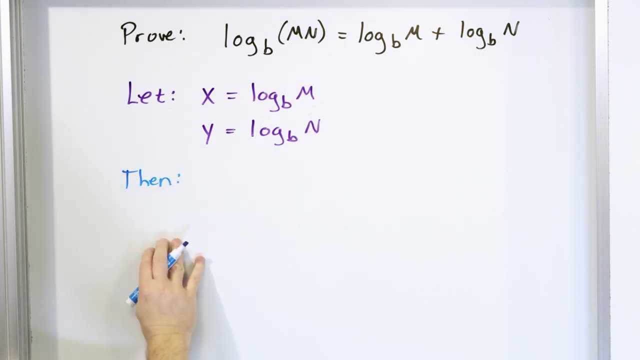 The rest of it. I'm going to try to logically connect the dots and make this thing be true. Okay, But if I let these things true, then the following things are true, because this is a logarithm. Then I then know because of this: 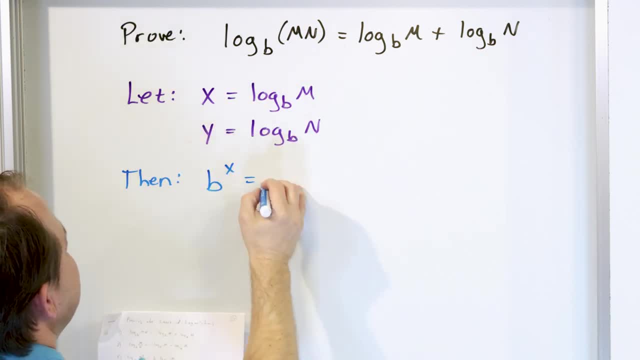 first line, b to the power of x is equal to m. b to the power of x is m. That's a definition of a logarithm. And also b to the power of y is equal to n. So because of what I let these variables 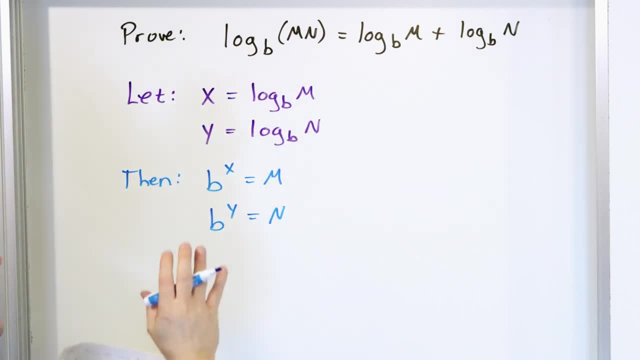 equal, then these variables are equal. You might say this is not at all looking like that. That's fine, That's what I said. You probably you know, unless you're a math you know guru, you probably wouldn't know to do this. I mean, none of us would. but as long as you can follow what I'm, 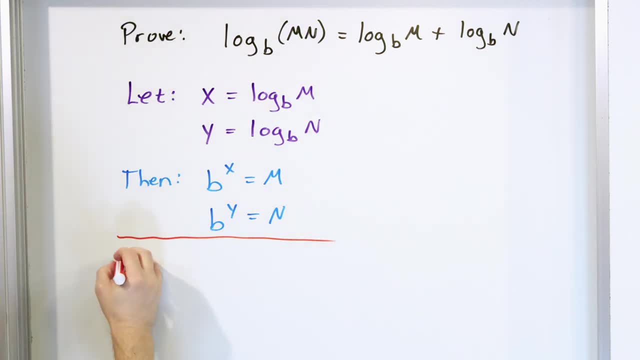 doing. that's all I care about. All right, Then. or I should say thus: you can use words like thus in a proof: If I let this true, then this become is true because of the definition of a logarithm, Then I know I want to multiply these things together m times n Okay, But now I know what. 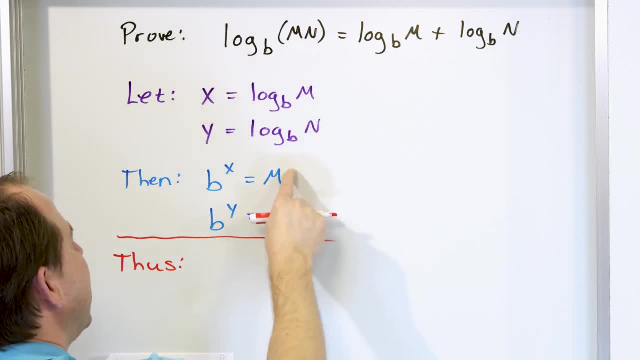 m and n are. They came from these definitions. You see, now I have equations for what m and n are. So then, m times, n is this times, which means that's b to the x, times, b to the y. You see, because I know what m and n are, 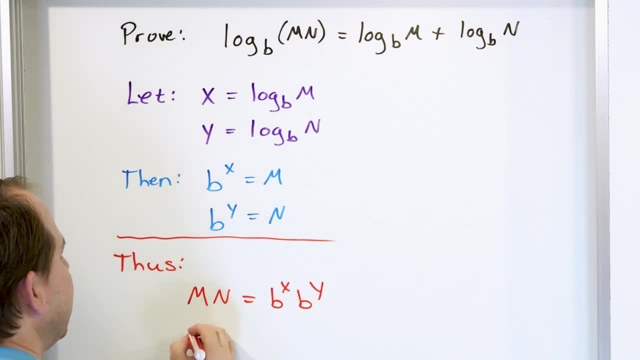 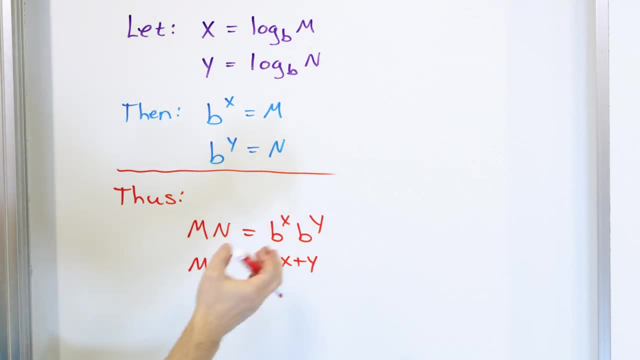 those things multiply together. But because these have the same base and different exponents, I can then say that this is b to the power of x plus y. because I can add these exponents Anytime. I have the same base, I can take those exponents there. I can add those exponents Now. ultimately, 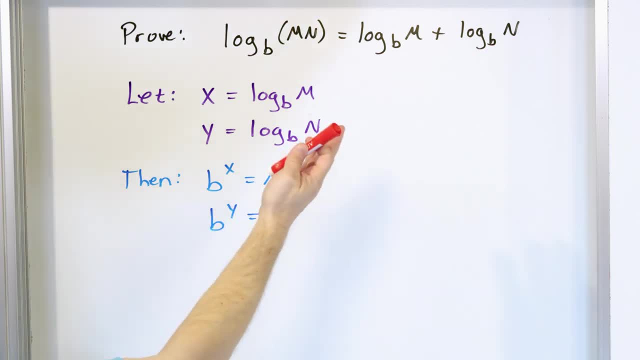 Probably you know. unless you're a math you know guru, you probably wouldn't know to do this. I mean, none of us would. But as long as you can follow what I'm doing, that's all I care about. 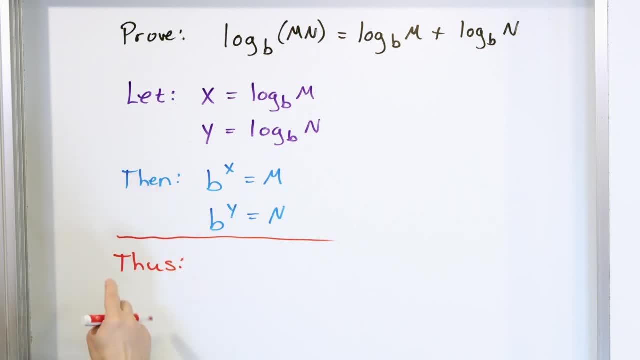 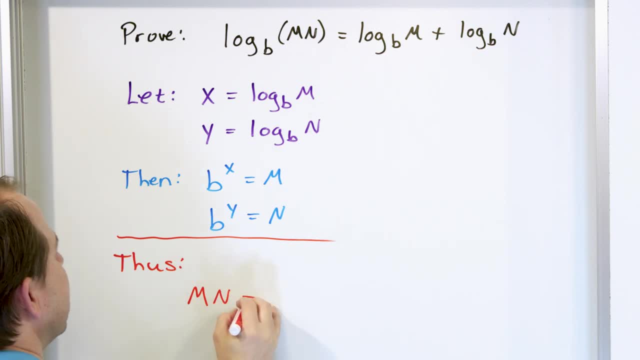 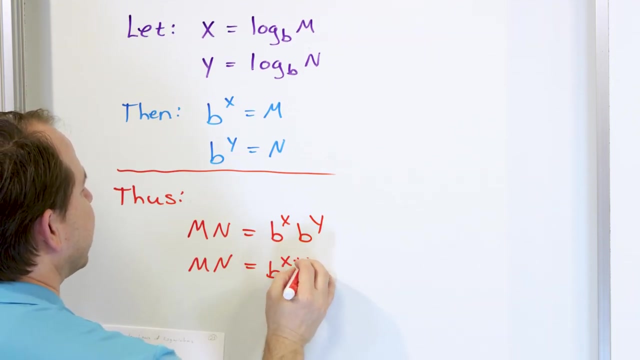 m and n are. So then m times n is this times this, which means that's b to the x times b to the y. You see, because I know what m and n are, those things multiply together, But because these have the same base and different exponents, I can then say that this is b to the power of x plus y. 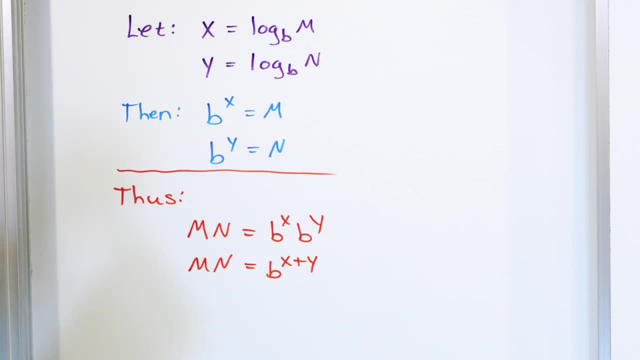 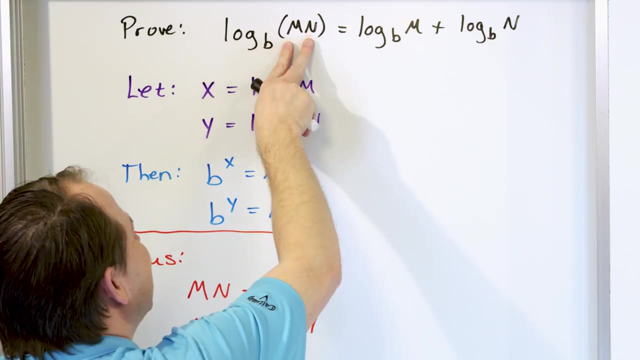 because I can add these exponents Anytime. I have the same base. I can take those exponents there. I can add those exponents Now. ultimately, I have m times n and I'm trying to take the logarithm of that and I want to see what it equals. Now I have an expression for what m times. 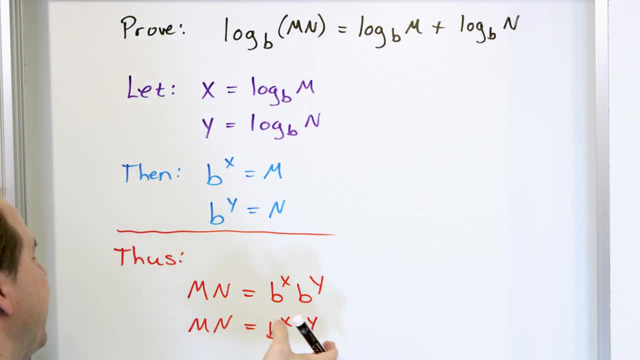 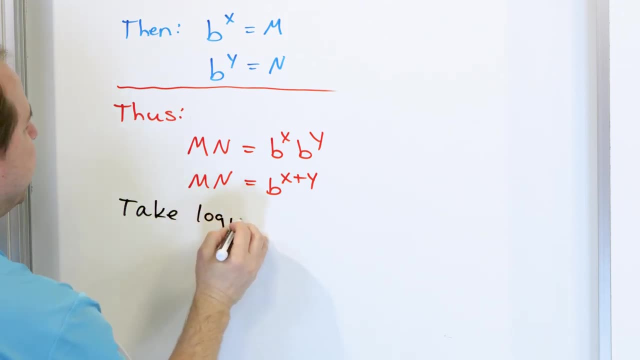 n actually is. So, in order to figure out if this is going to work out, I'm going to take logarithm of both sides. So I'll take log of base b, both sides, because I can do anything I want to an equation as long as I do it to both sides. So I'm going to work with this one. I'm going to say log. 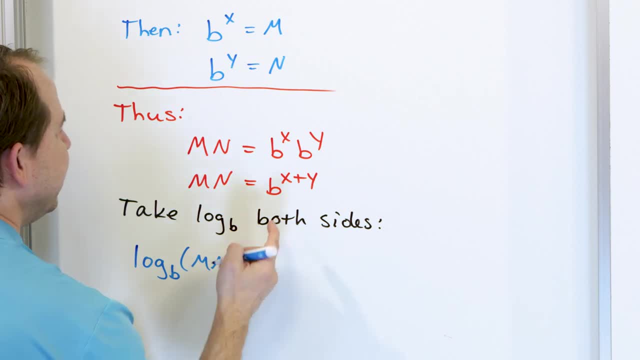 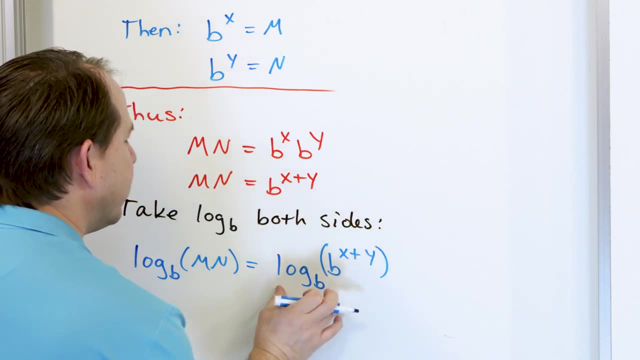 base b of m times n is equal to. I'm going to have to take the log of this log: base b of b to the power of x plus y. Now, this b to the power of x plus y, this is what the 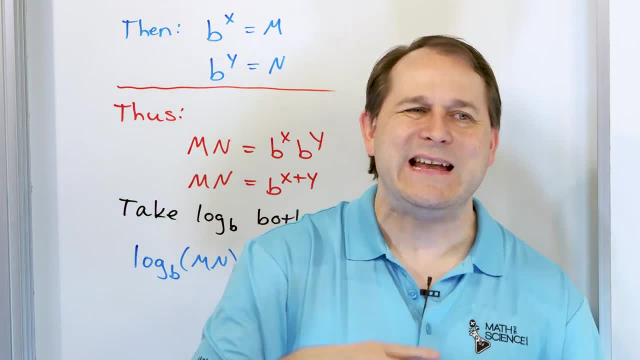 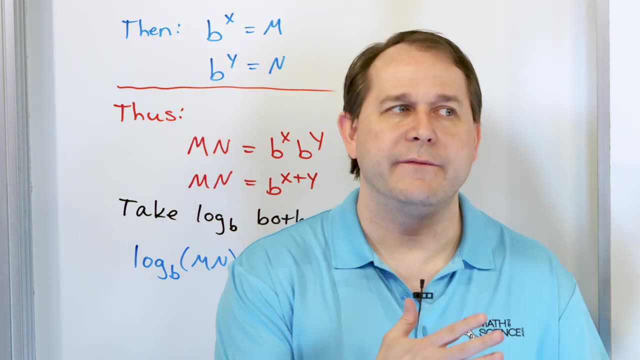 logarithm is operating on. But remember we talked about 90 million times about the idea that a logarithm with a base b is the inverse function of an exponential with a base b. They're inverses, So when they operate on each other, they annihilate each other. That is what the definition of the 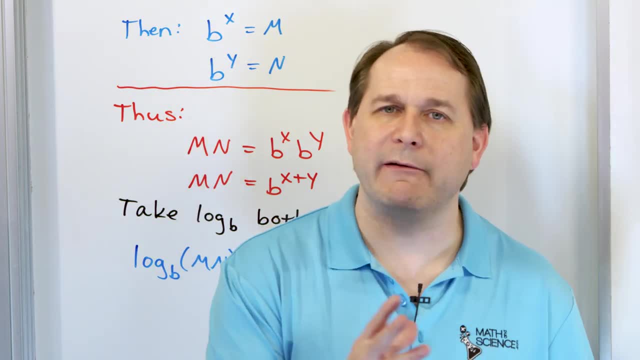 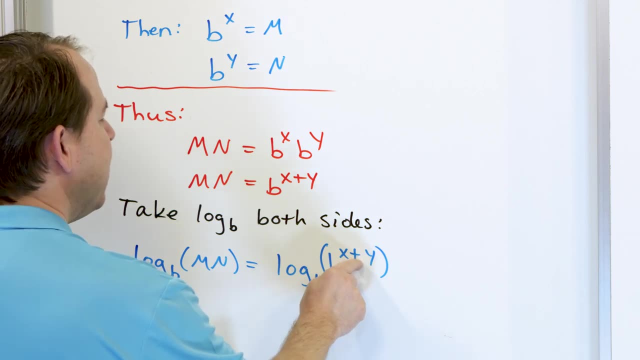 inverse does. The inverse function undoes what the parent function or what the other function did in the first place. So since we have an exponential, we have an inverse function. So we have an exponential here. It raised to the power b, to the power of this, but the logarithm. 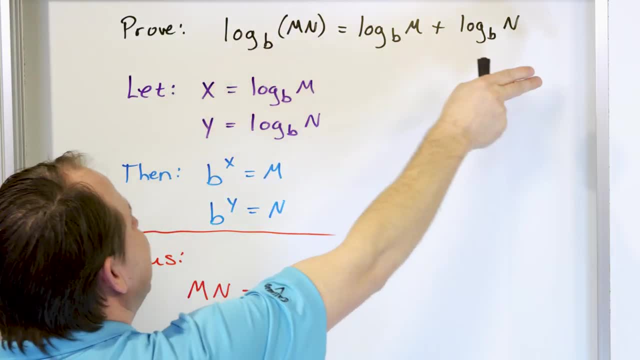 I have m times n and I'm trying to take the logarithm of that and I want to see what it equals. Now I have an expression for what m times n is, So I'm going to take the logarithm of that. 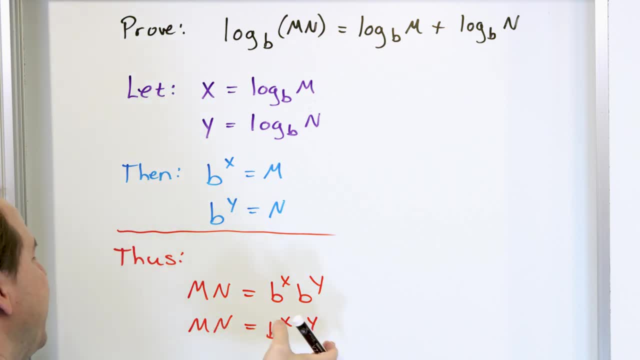 and I'm going to see what it equals. Now I have an expression for what m times n is, So I'm going to actually is So. in order to figure out if this is going to work out, I'm going to take logarithm. 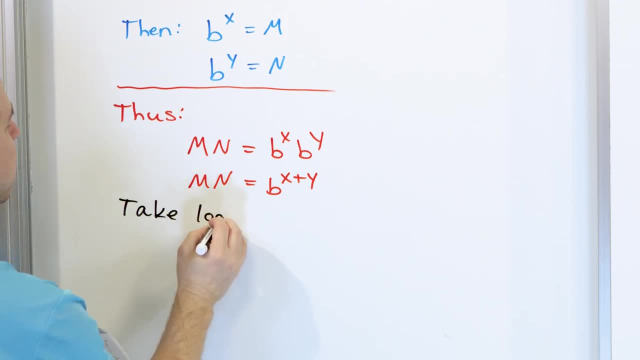 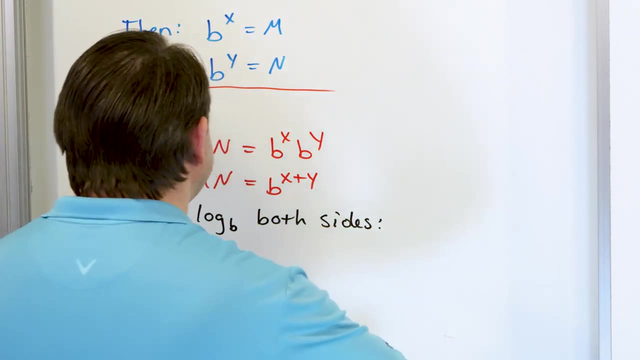 of both sides. So I'll take log of base b, both sides, because I can do anything I want to an equation as long as I do it to both sides. So I'm going to work with this one. I'm going to say log. 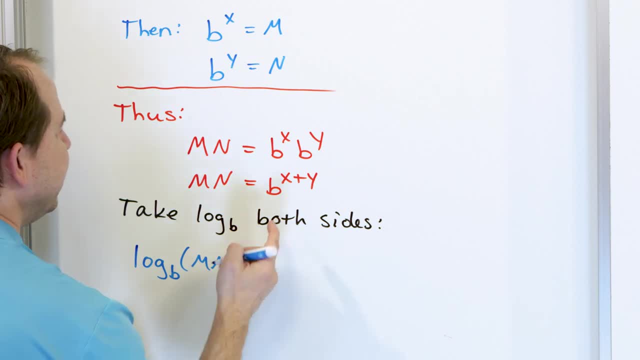 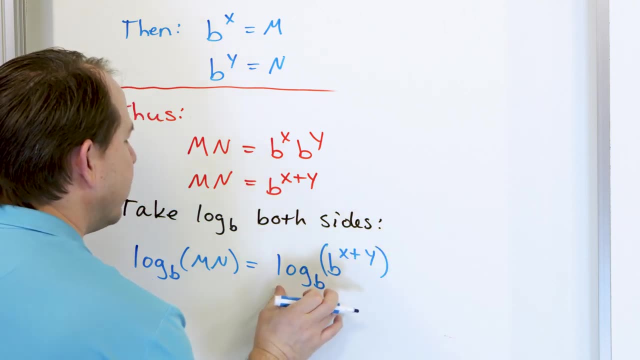 base b of m times n is equal to. I'm going to have to take the log of this log: base b of b to the power of x plus y. Now, this b to the power of x plus y. this is what the logarithm is operating on, But remember we talked about 90 million times. 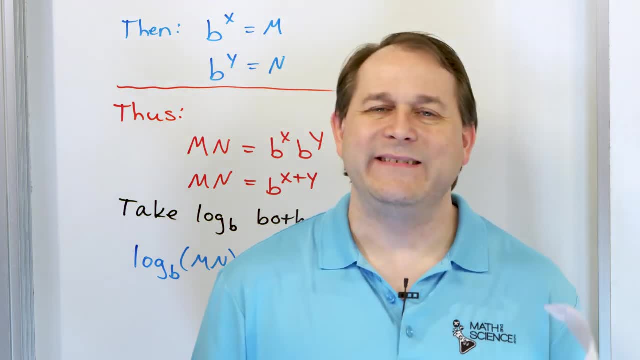 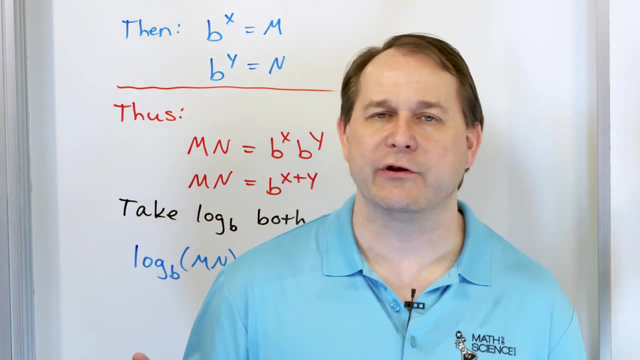 about the idea that a logarithm with a base b is the inverse function of an exponential with a base b. They're inverses, So when they operate on each other they annihilate each other. That is what the definition of the inverse does. The inverse function undoes what the parent function or what 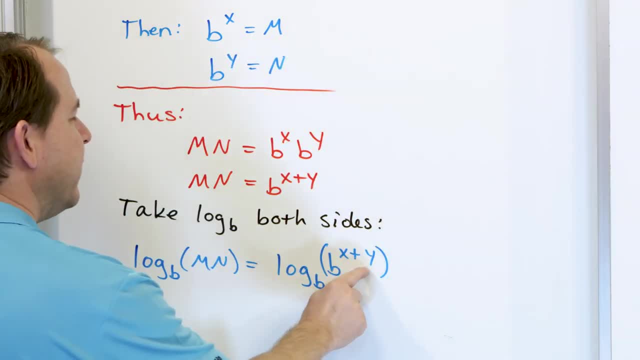 the other function did in the first place. So, since we have an exponential here, it raised to the power b, to the power of this, but the logarithm undoes that. So we have an exponential that. So on the right-hand side, the logarithm cancels with the base b and all I have left is x. 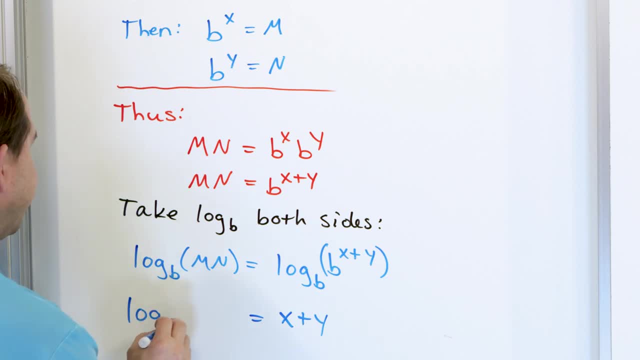 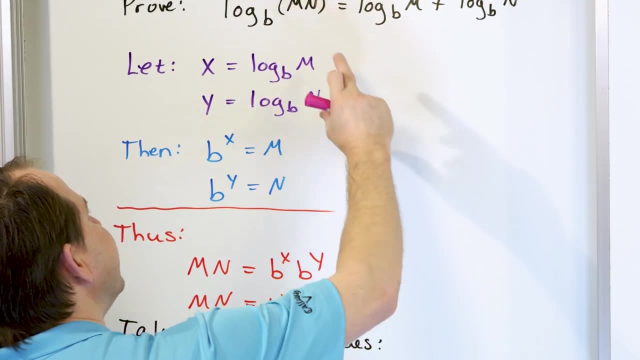 plus y. On the left-hand side I have the logarithm base b of m times n. So you might say, great, but I don't care about x plus y. But then you remember, wait a minute- I defined what x and. 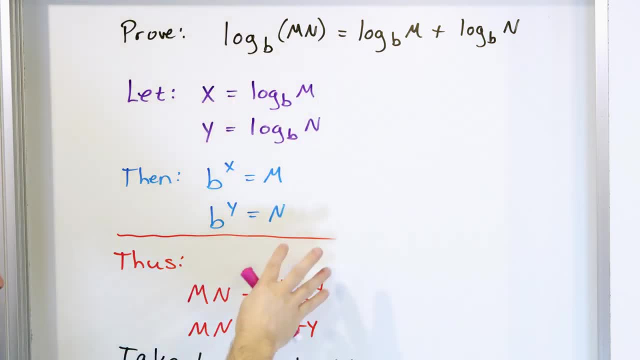 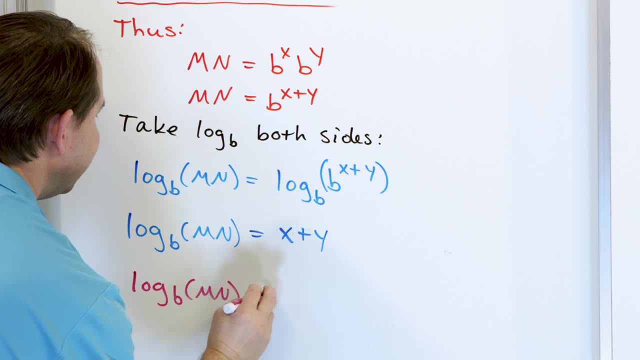 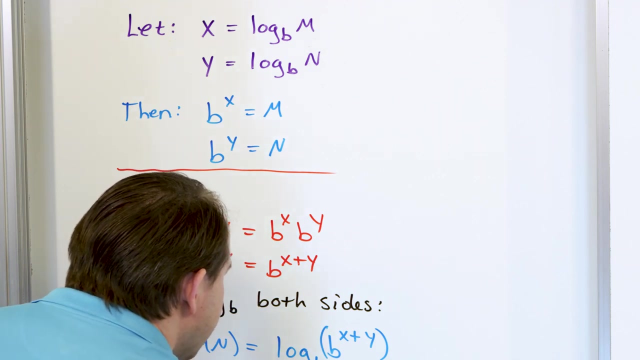 y were up here. This x and y are the same ones that are rippling through the problem statement. So then you know that the logarithm base b of m times n is equal to x, but x is the logarithm base b of m. Log base b of m. There's a plus sign here, Why? Why is log base b of m? 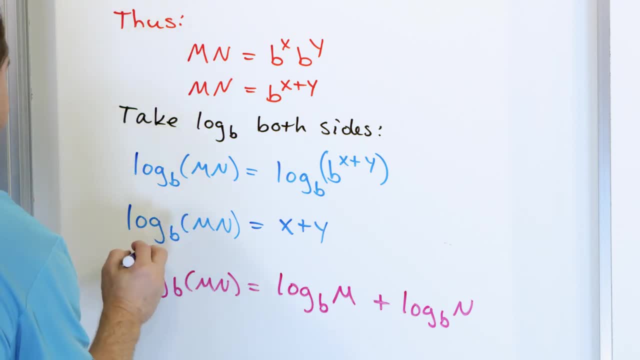 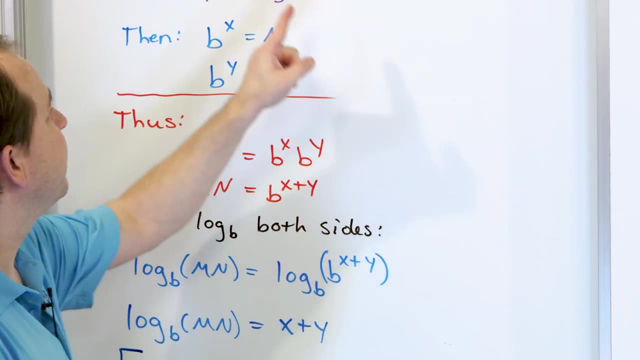 And if you look back and compare these things, these are exactly the same thing. All right, because log base b of the product becomes the logarithm of the first one plus the logarithm of the second one. That's exactly what we set out to prove. Do I expect that you? 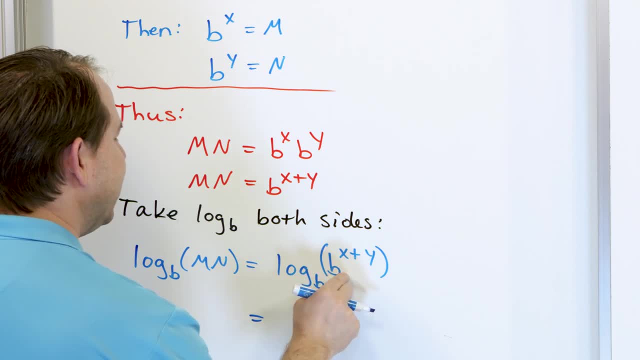 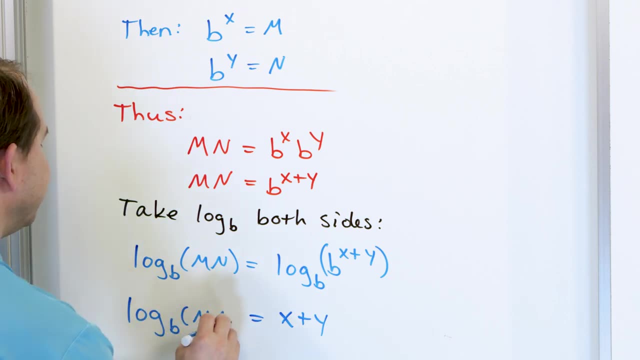 undoes that. So on the right-hand side the logarithm cancels with the base b and all I have left is x plus y. On the left-hand side I have the logarithm base b of m times n, So you might. 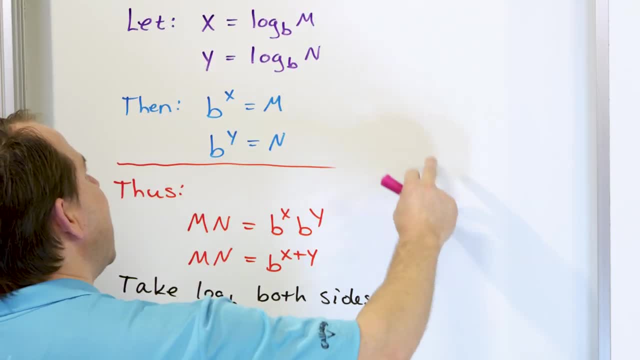 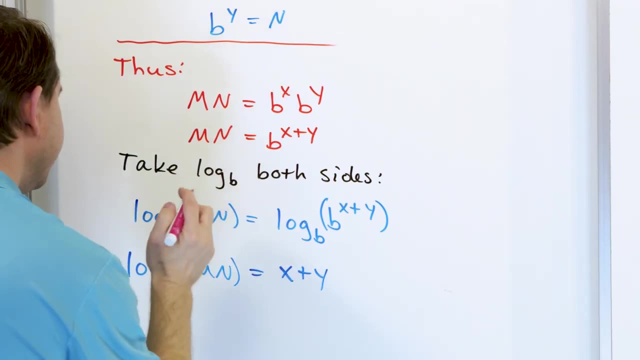 say great, but I don't care about x plus y. But then you remember- wait a minute- I defined what x and y were up here. This x and y are the same ones that are rippling through the problem statement. So then you know that the logarithm base b. 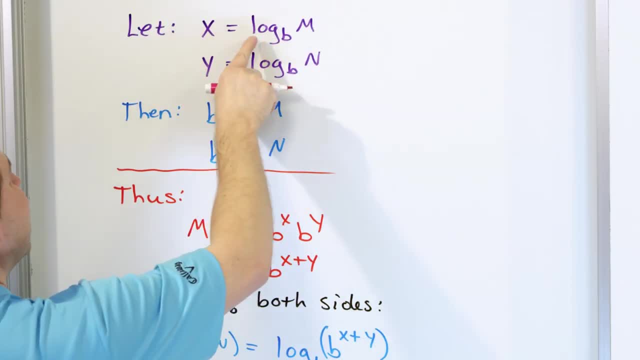 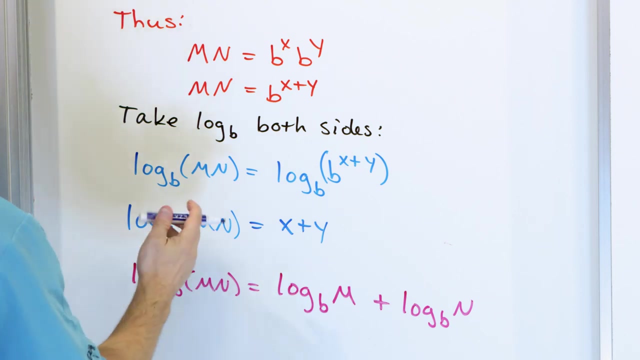 of m times n is equal to x, but x is the logarithm base b of m, Log base b of m. There's a plus sign here- y. y is log base b of n And if you look back and compare these things, these are exactly. 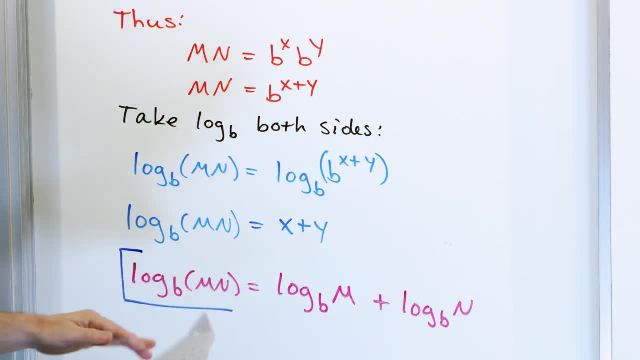 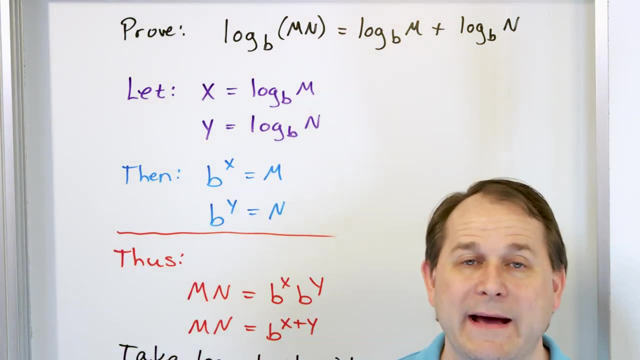 the same thing. All right, because log base b of the product becomes the logarithm of the first one plus the logarithm of the second one. That's exactly what we set out to prove. Do I expect that you would have known how to do that? 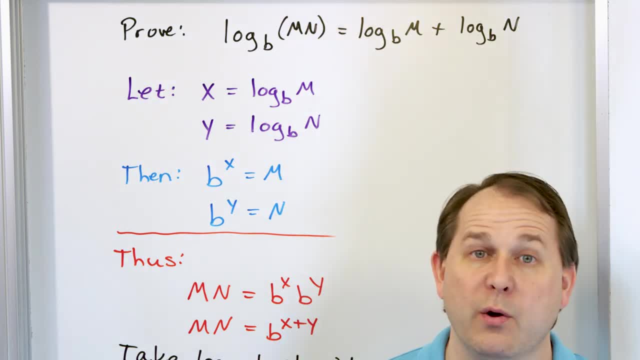 No, Most teachers are not going to tell you prove the first law of logarithms. But what does it do? It allows you to understand how to get this from the definition That's a property of logarithms. When you multiply them, you add exponents. When I take the log of both sides, the annihilation that 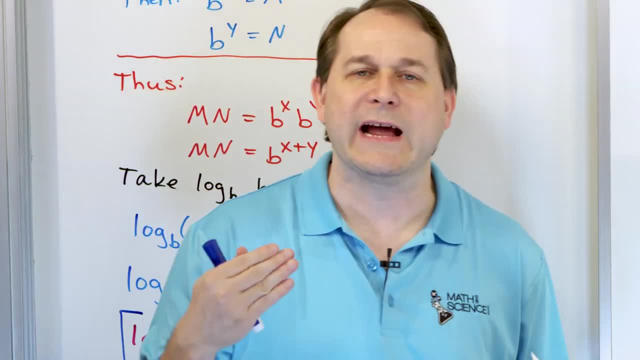 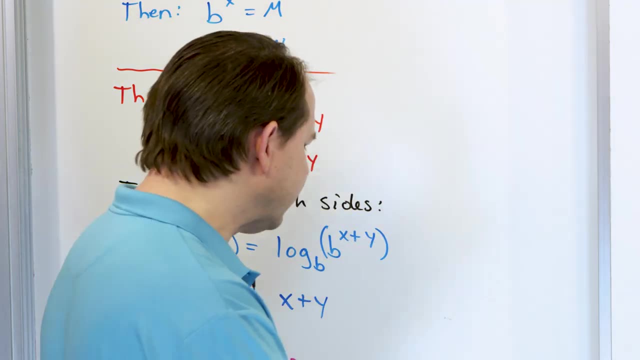 happens here. that's a property of logarithms. So in the process of learning how to prove these things, you actually sharpen your skills with dealing with logs. That's really all I care about in this lesson. Okay, Let's go ahead and prove the. 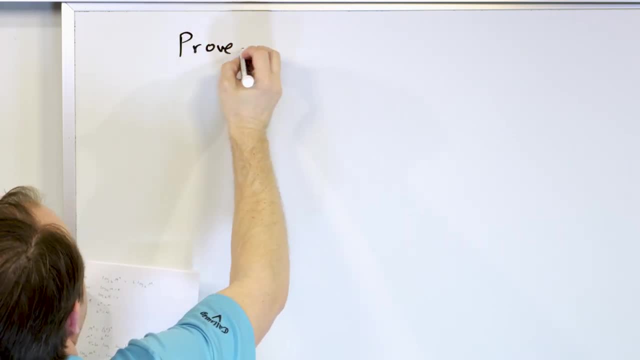 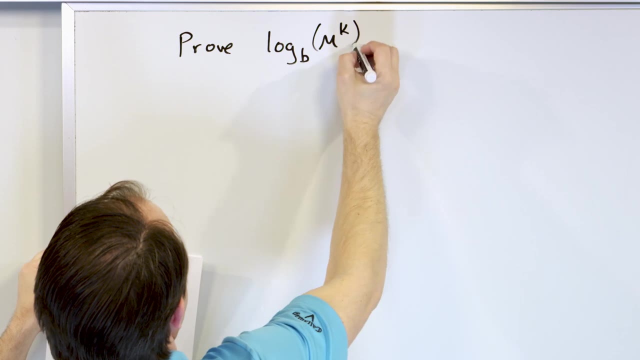 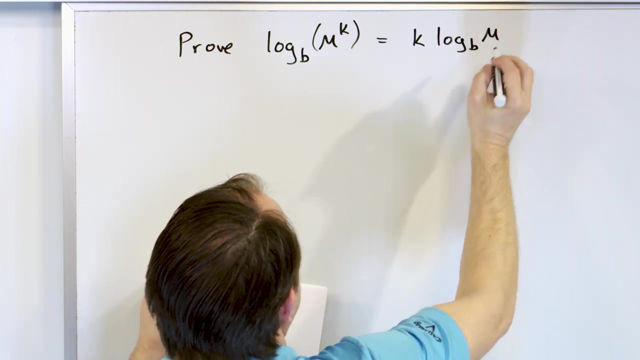 one about exponents next. So we're going to prove log base b of m to the power of k, some number to the power of k, And we know that that's equal from our laws of logarithms to k. log b of m like. 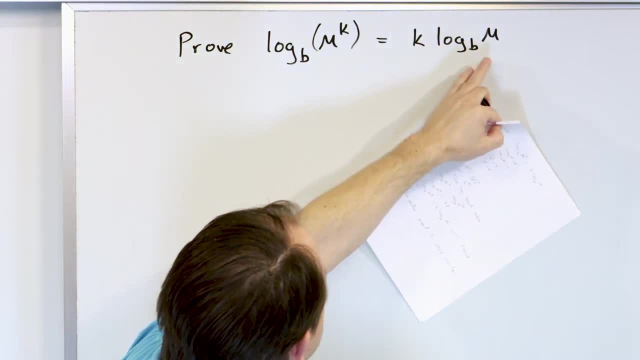 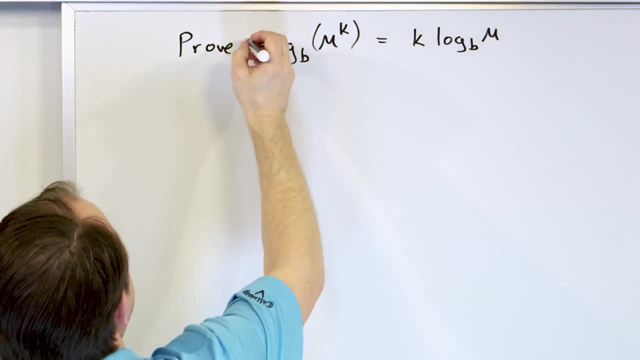 that, Okay, k log b, base b of the number m. So basically, we can take an exponent, we can bring it out in front of the logarithm. That's all this is telling us. How do we prove that? So we need to. 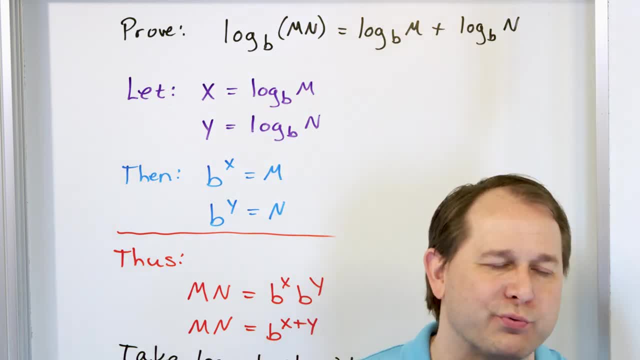 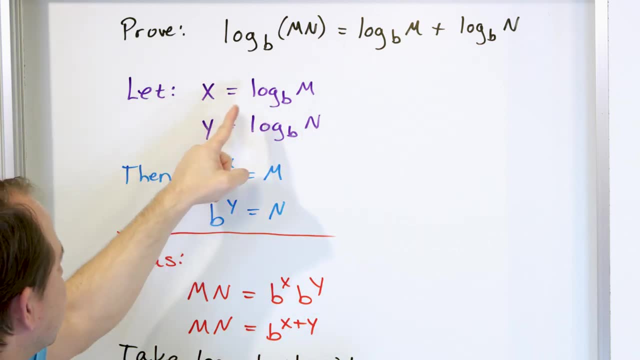 would have known how to do that. No, Most teachers are not going to tell you prove the first law of logarithms. But what does it do? It allows you to understand how to get this from the definition That's a property of logarithms. 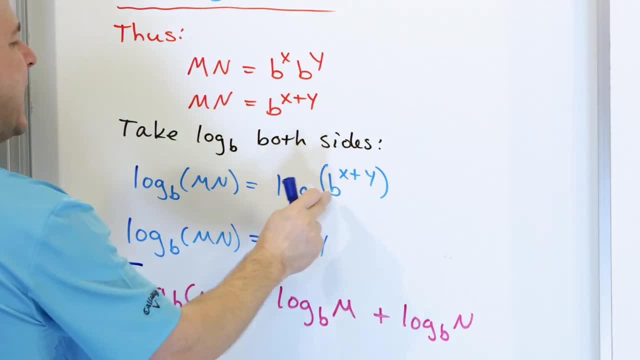 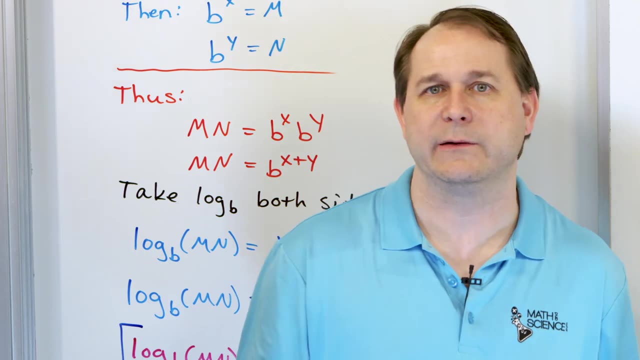 When you multiply them, you add exponents. When I take the log of both sides, the annihilation that happens here, that's a property of logarithms. So in the process of learning how to prove these things, you actually sharpen your skills with dealing with logs. That's really all I care about. 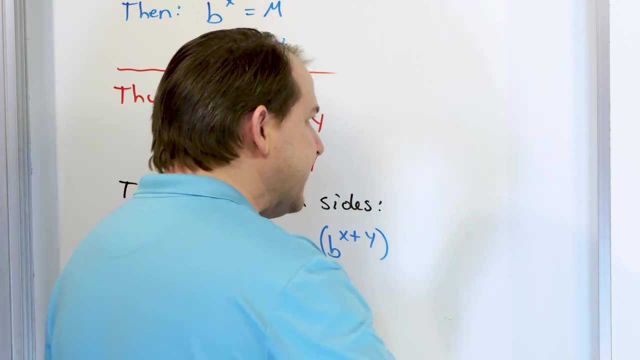 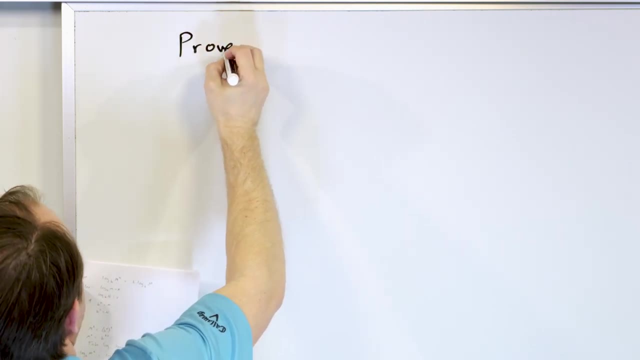 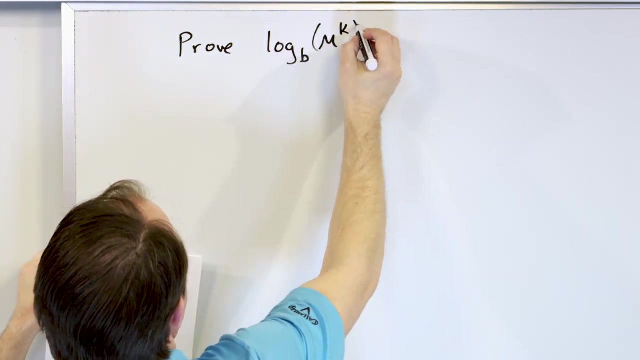 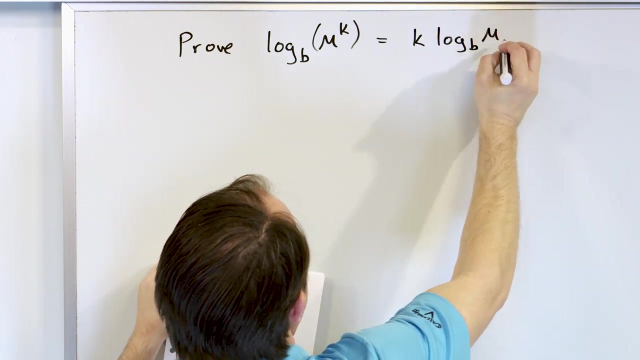 in this lesson. Let's go ahead and prove the one about exponents next. So we're going to prove that we have a logarithm of k log base b of m to the power of k, some number to the power of k, And we know that that's equal from our laws of logarithms to k log b of m, like that. 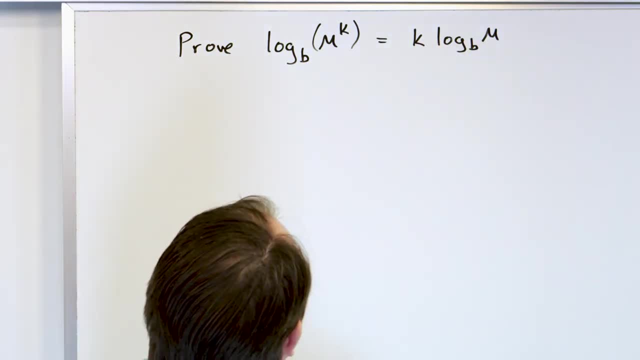 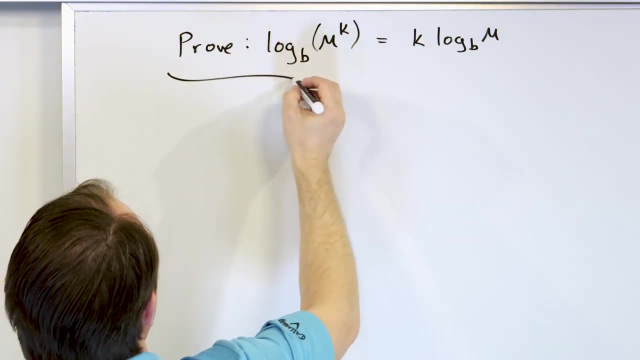 k, log b, base b of the number m. So basically, we can take an exponent, we can bring it out in front of the logarithm. That's all this is telling us. How do we prove that? So we're going to do the similar kinds of assumptions. We're going to have to let some things happen. 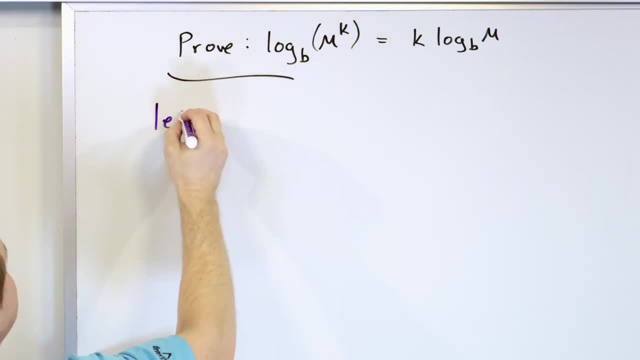 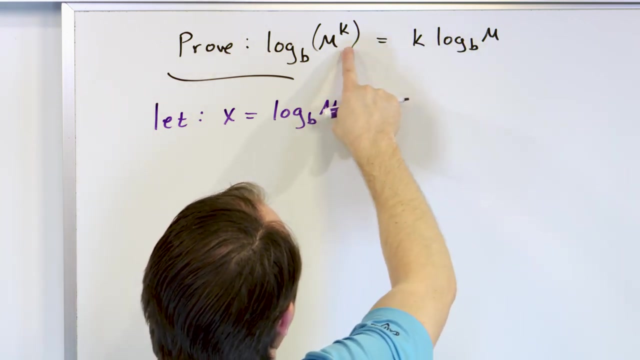 happen In this case. we're going to let x equal to log b of n. Now we could let y equal to log b of n, but you see, in this property of logs there is no n anywhere else. So we don't really. 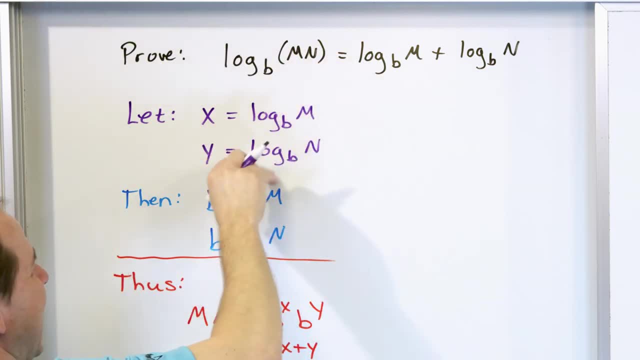 need to define that. Here we had an m and an n, so we had to kind of have a term for each one of them. But here there is no n anywhere, so there's no reason to really do that. But from this single. 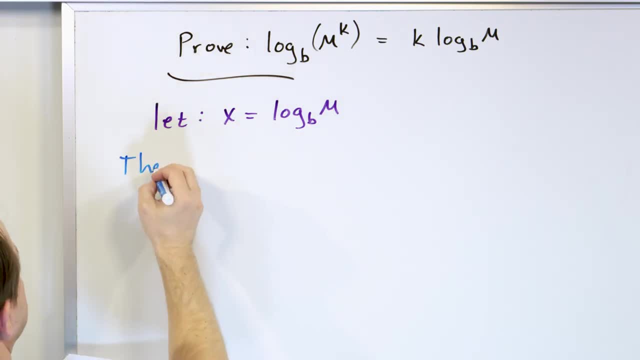 definition. here something pops out. The same exact thing as before. b to the power of x is equal to m. So so far it's just a rewrite of what we did on the other board, But we have a conclusion that we can draw here. I should say thus: right, Ultimately, what do I want? I want. 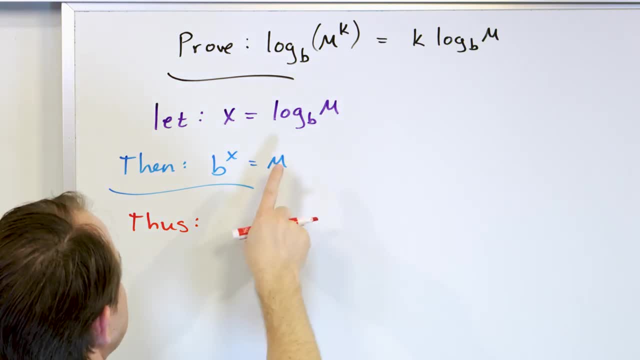 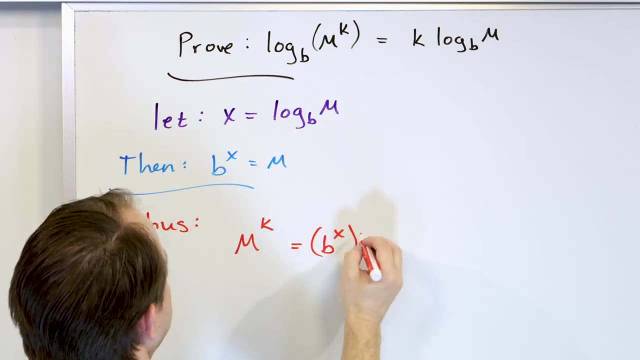 m to the power of k. okay, m to the power of k. So this thing, m to some power of k is what's on this side, b to the x raised to the sum power of k. All I've done is I said hey. 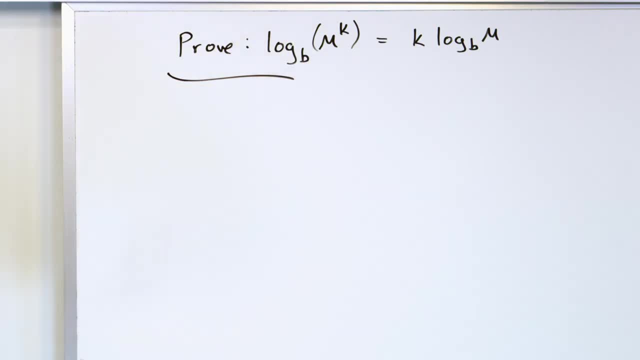 do we're going to do the similar kinds of assumptions. Okay, We're going to have to let some things happen. Okay, In this case we're going to let. we're going to let x equal to log b of m. Okay, Now we could let y equal to log b of n. but you see, in this property of logs, 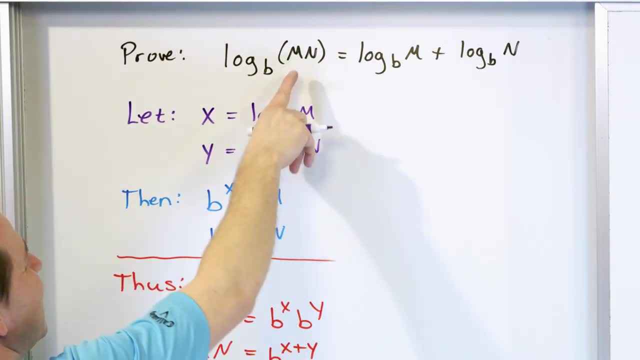 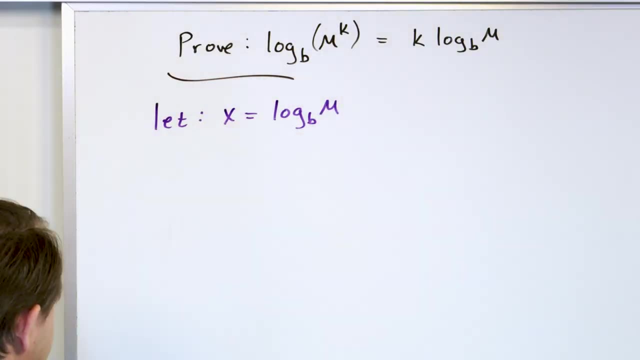 there is no n anywhere else, So we don't really need to define that. Here we had an m and an n, so we had to kind of have a term for each one of them, But here there is no n anywhere, So there's no reason to really do that. But from this single definition here 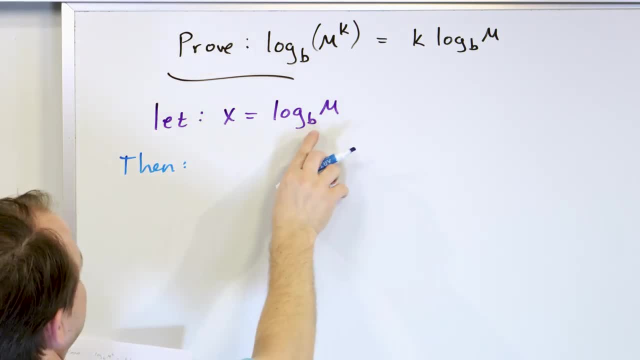 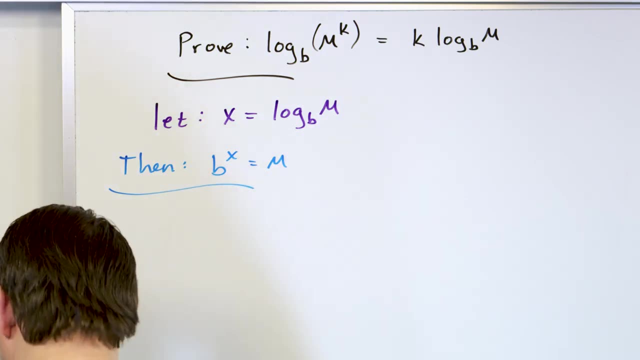 something pops out, The same exact thing as before: b to the power of x is equal to m. So so far it's just a rewrite of what we did on the other board, But we have a conclusion that we can draw here. I should say thus: right, Ultimately, what do I want? I want m to the power of k. Okay, 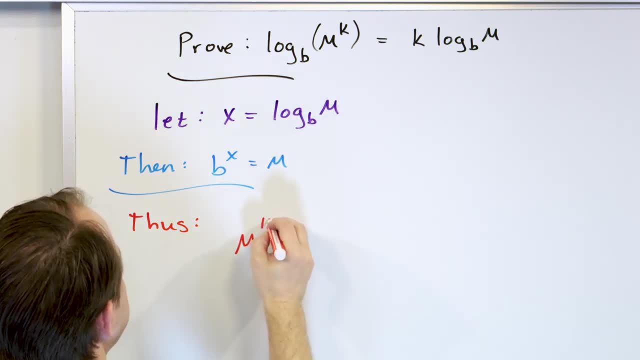 Okay, So this thing, m to some power of k, is what's on this side, b to the x raised to the sum power of k. All I've done is I said, hey, this gives me a definition for what m is. I want to. 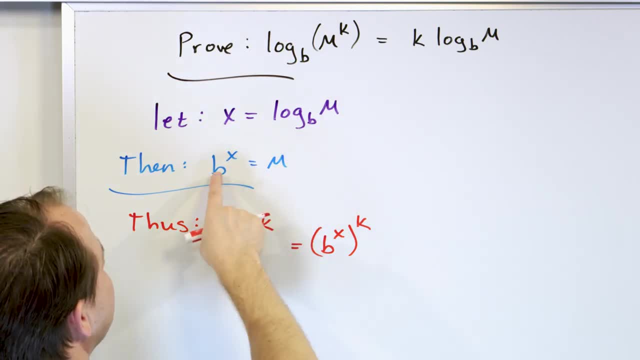 raise it to a power because that's what's in my proof. So I raise it to a power. so I have to raise this side to the power because that's what it's equal to. But this means that m to the power. 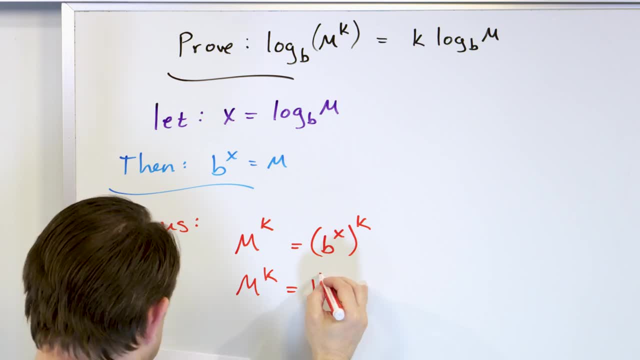 of k is b to the. how do I want to write it? kx, Because this is an exponent raised to an exponent. so I'm going to multiply those things. So I'm going to multiply those things and I'm going to. 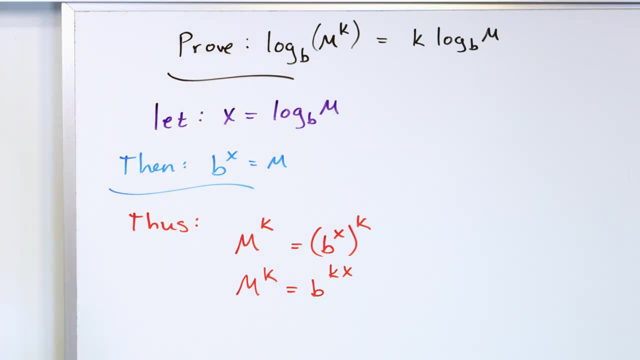 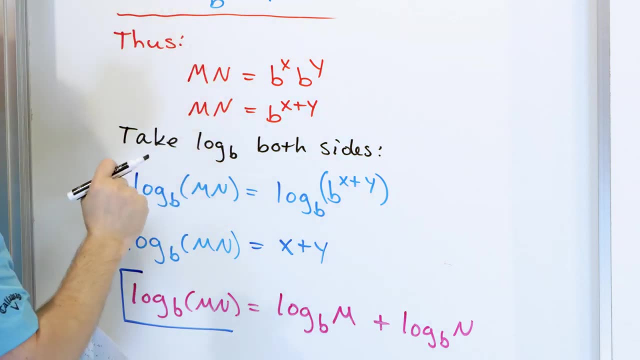 The sum of m is a product of natural reduction. So I'm going to make sure that I get the proper things together. And what did we do in the last thing? Once we had it all kind of written out like this, we wanted to get m times n to match our problem statement. Here we have m to the power of. 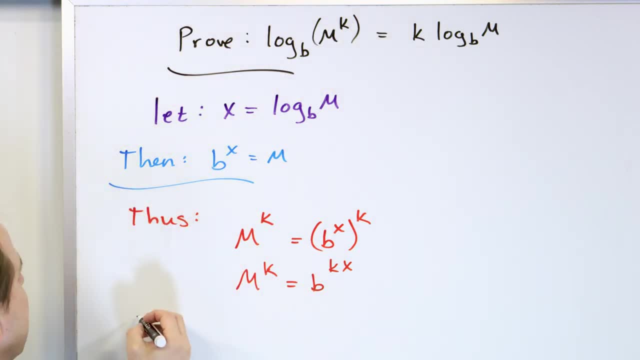 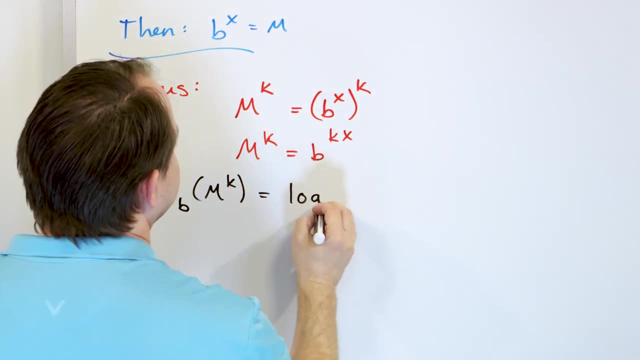 k to match what's in our proof. so now we want to take log of both sides, So we'll take the logarithm. We'll take a base b, logarithm of m to the power of k, logarithm, base b of what's on the. 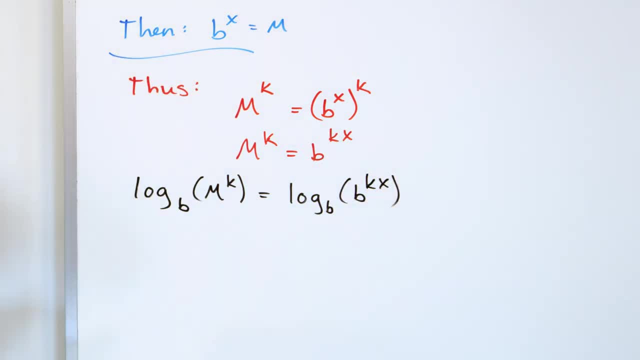 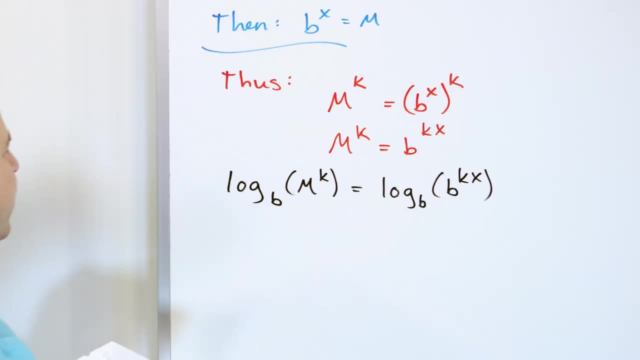 right-hand side b to the power of kx like this, But then you know that on the right-hand side you're going to get the same annihilation. here You have a log of an exponent. Those two things are going to cancel. just like we had a log of an exponential, here We have a log of an exponential. 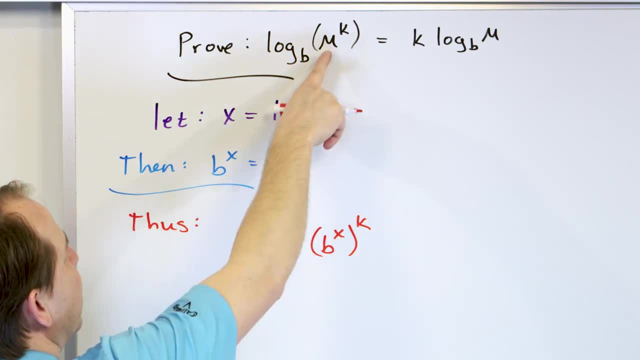 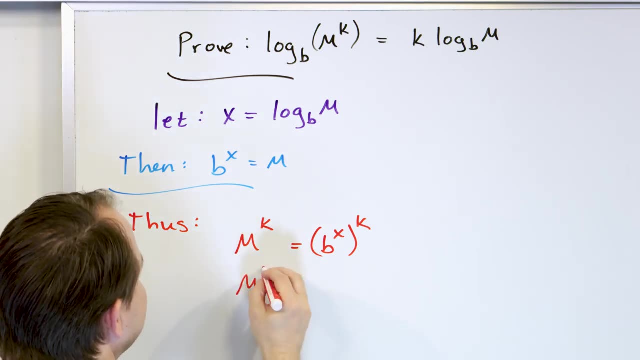 this gives me a definition for what m is. I want to raise it to a power because that's what's in my proof. So I raise it to a power. so I have to raise this side to the power because that's what it's equal to. But this means that m to the power of k is b to the. how do I want to write it? kx. 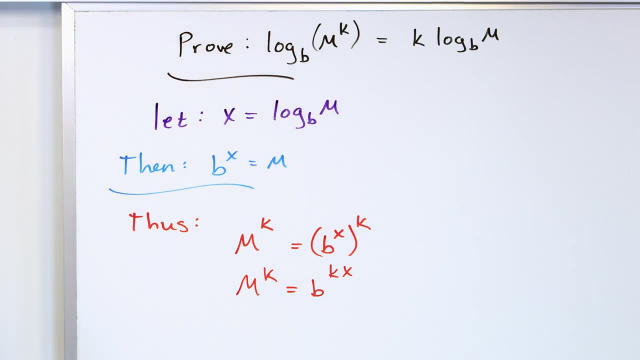 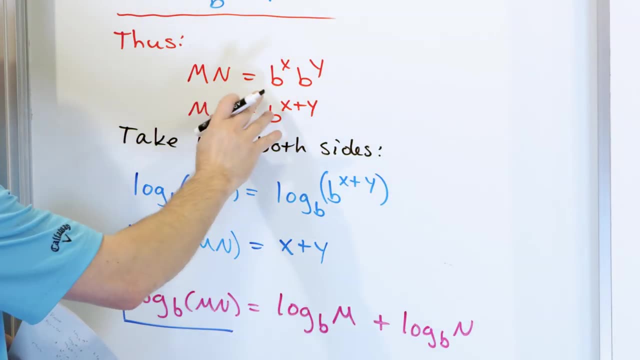 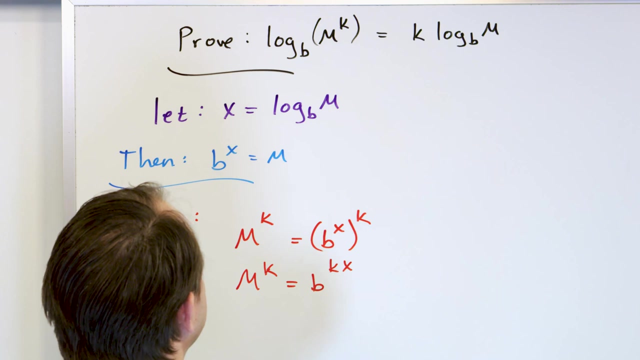 because this is an exponent raised to an exponent. So I'm going to multiply those things together. All right, What did we do in the last thing? Once we had it all kind of written out like this: we wanted to get m times n to match our problem statement. Here we have m to the power of k to match what's in our 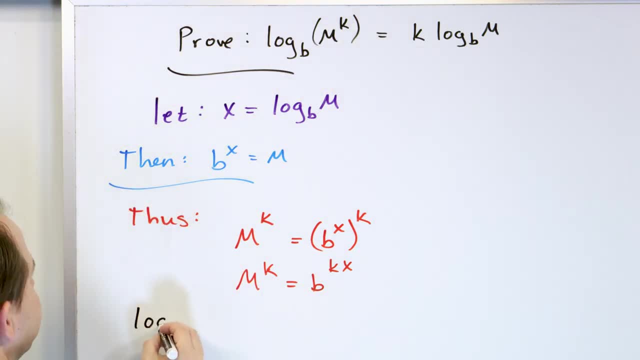 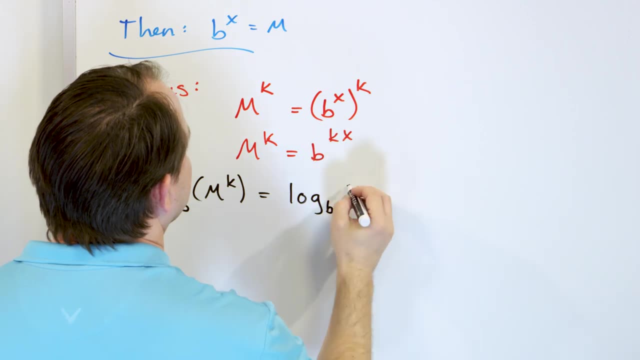 proof. So now we want to take log of both sides, So we'll take the logarithm. We'll take a base b, logarithm of m to the power of k. logarithm, base b of what's on the right-hand side, b to the power. 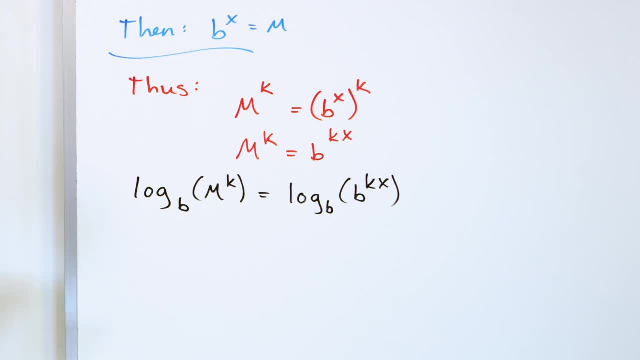 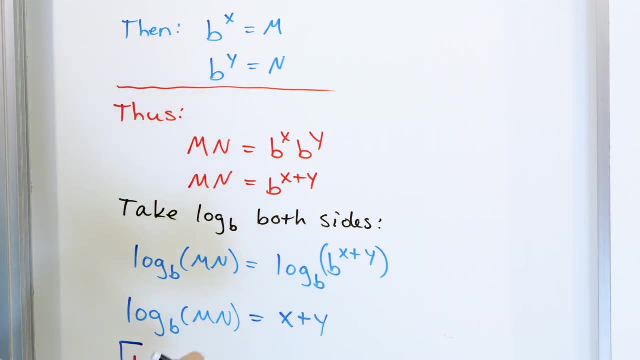 of kx like this, But then you know that on the right-hand side you're going to get the same annihilation. here You have a log of an exponent. Those two things are going to cancel, just like we had a log of an exponential. 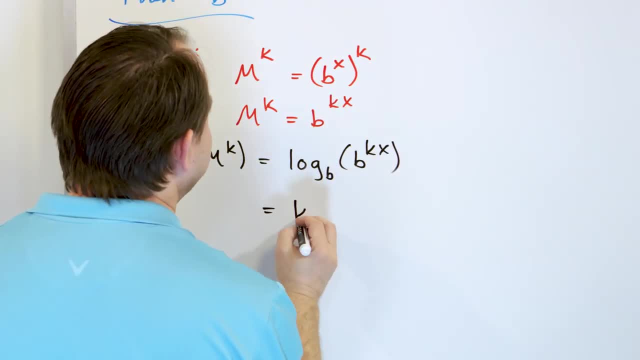 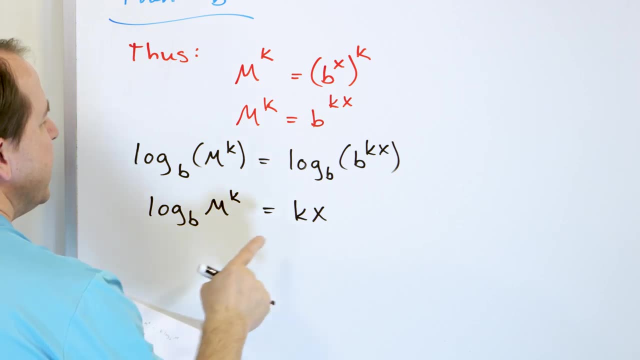 here We have a log of an exponential here On the right-hand side. all you're going to have is k times x. On the left-hand side you're going to have log base b of m to the power of k And you. 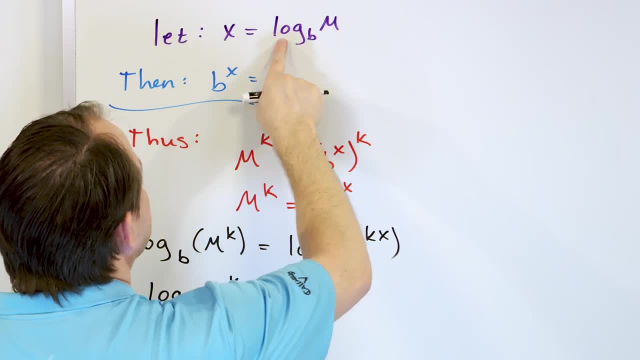 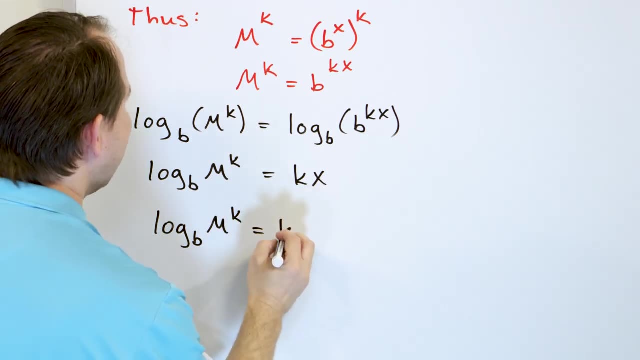 have k times x And you say, well, wait a minute, I know what x is. X was log base b of m, So you're going to have log base b of m to the power of k. is k multiplied by x? But I know what that is. It's. 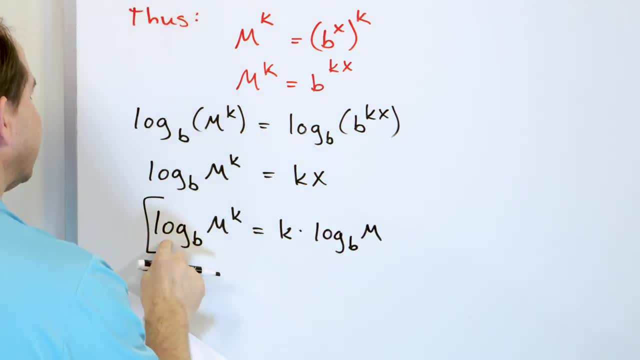 log base b of m. So that's the way that we're going to do it, And then we're going to minimize work base b of m. You see, you take the logarithm of something with an exponent. you could just take that exponent right out front and then multiply by the log of that base there. 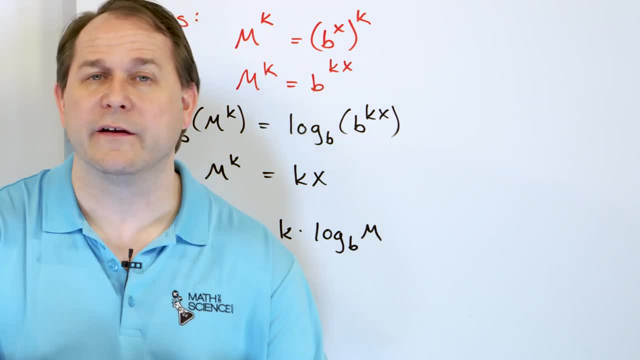 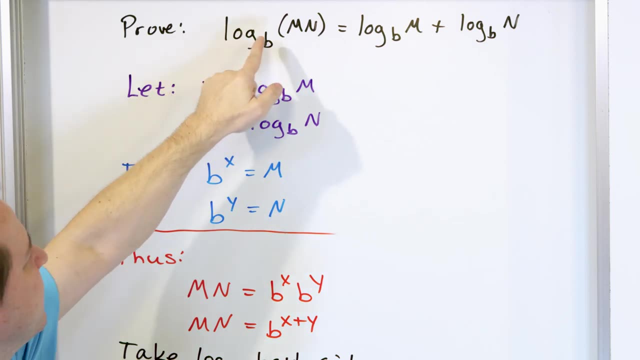 So that is the proof of one of the three laws of logarithms, the one that deals with exponents. Now, the one that I say for last is the one that looks kind of like this: Remember, there's one that talks about multiplying things becomes addition of logs. and then there's another. 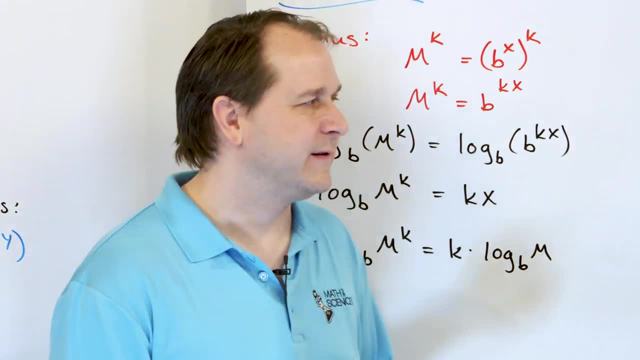 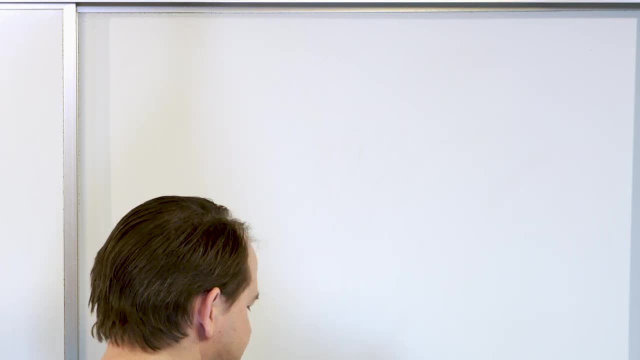 one that talks about division of things becomes subtraction of logs. So our last one that we're going to do- and this would be the last thing we'll prove in this lesson- is: we want to prove. Let me flip my page here just to make sure I don't mess anything up. Let's 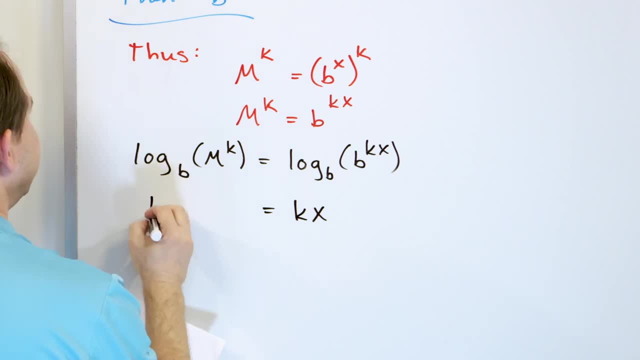 here On the right-hand side, all you're going to have is k times x. On the left-hand side, you're going to have log base b of m to the power of k And you have k times x and you say: 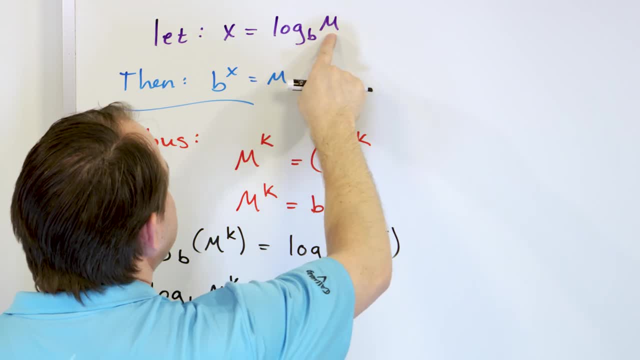 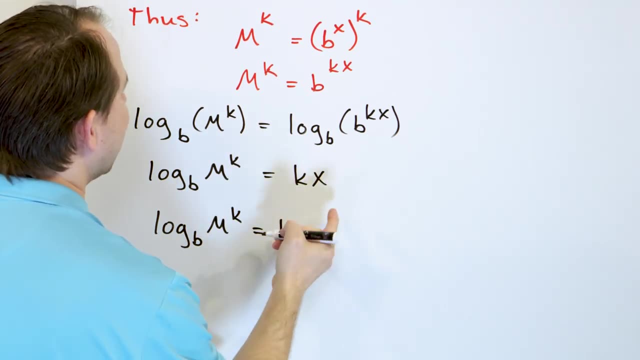 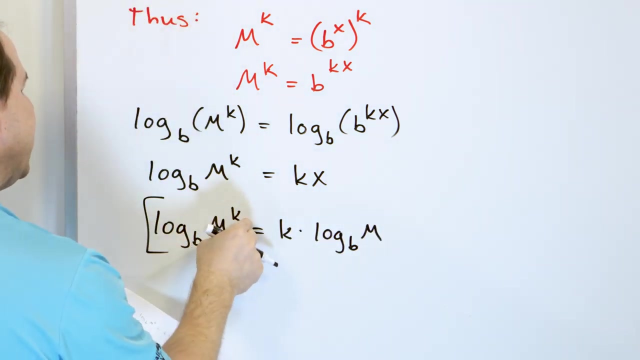 well, wait a minute. I know what x is. x was log base b of m, So you're going to have log base b of m to the power of k is k multiplied by x? but I know what that is: It's log base b of m. You see, you take the logarithm of something with an exponent. 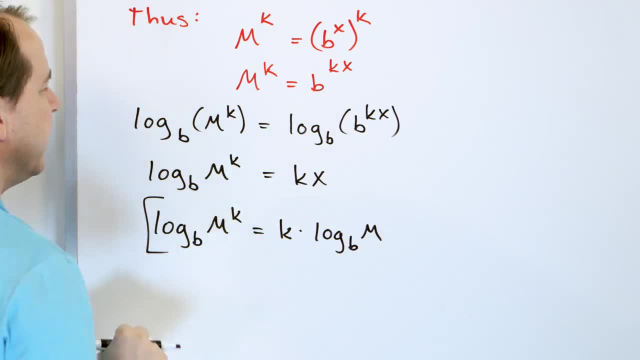 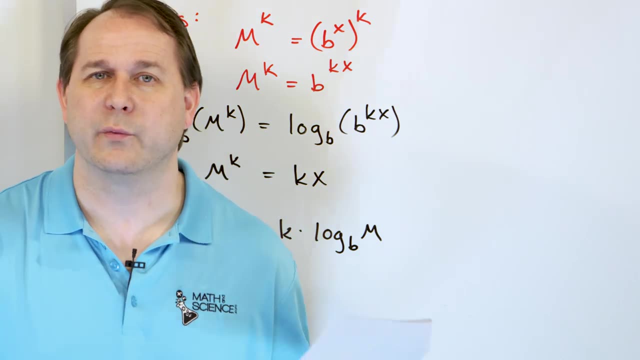 You can just take that exponent right out front and then multiply by the log of that base there. So that is the proof of one of the three laws of logarithms, the one that deals with exponents. Now, the one that I say for last is the one that looks kind of like this: Remember, there's one that talks: 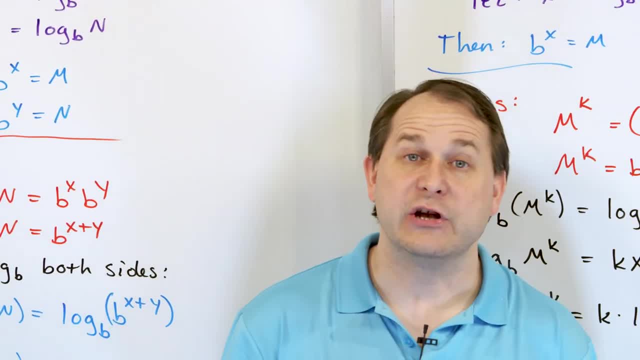 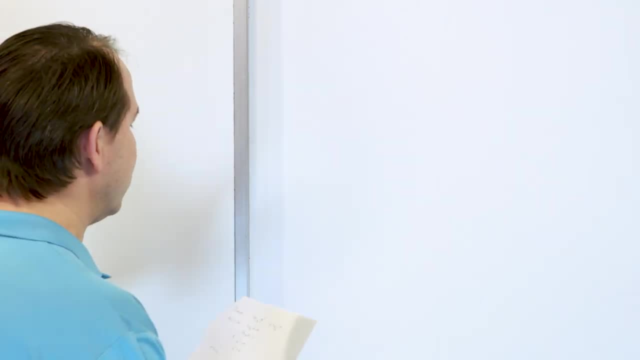 about multiplying things becomes addition of logs. and then there's another one that talks about division of things becomes subtraction of logs. So our last one that we're going to do- and this will be the last thing we'll prove in this lesson- is: we want to prove 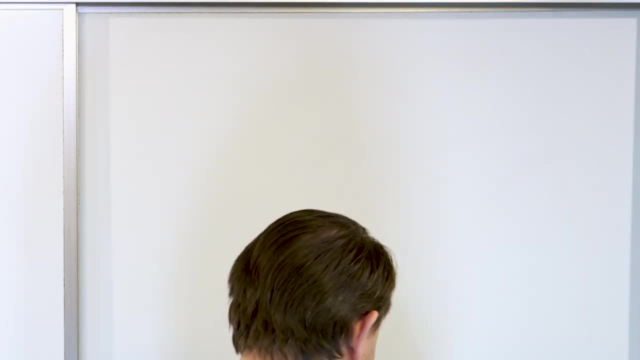 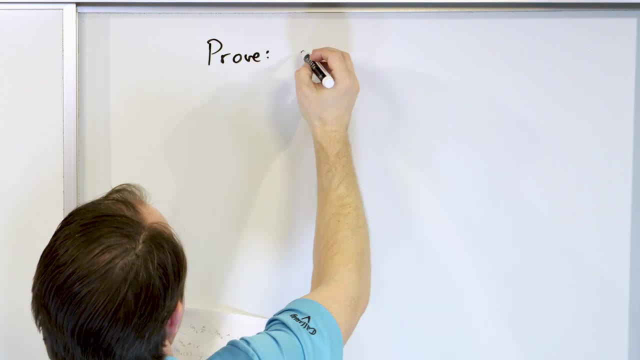 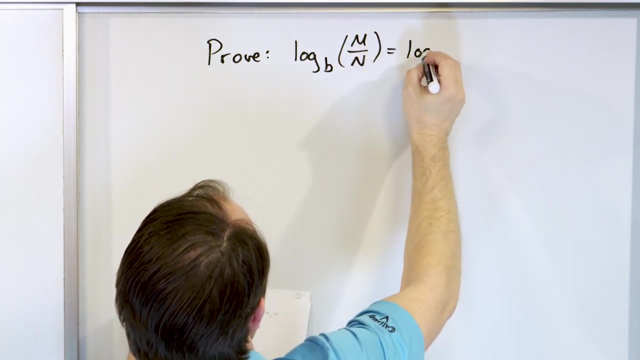 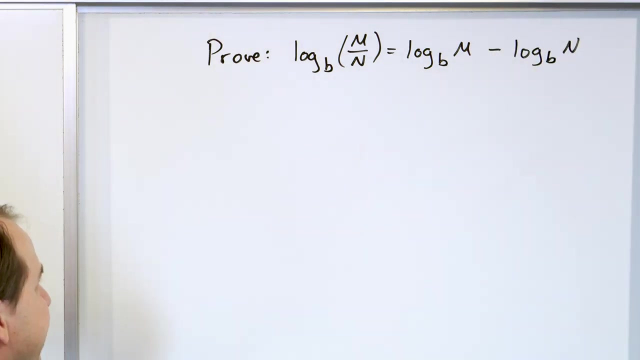 Let me flip my page here, just to make sure I don't mess anything up. Let's prove this last one. Prove the following thing: Log base b of the division m over n is equal to log base b of m minus sine log base b of n. So I want to do the subtraction there. 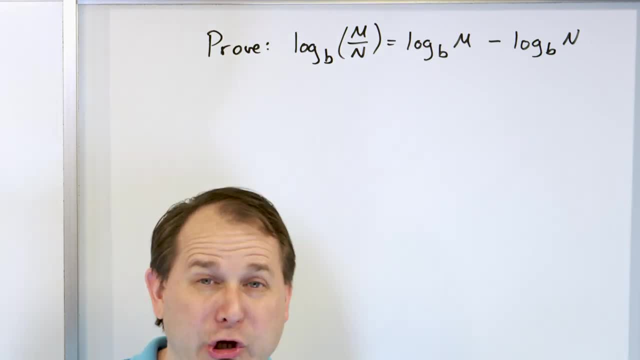 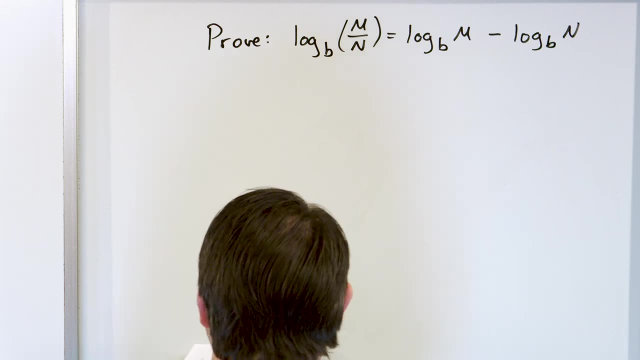 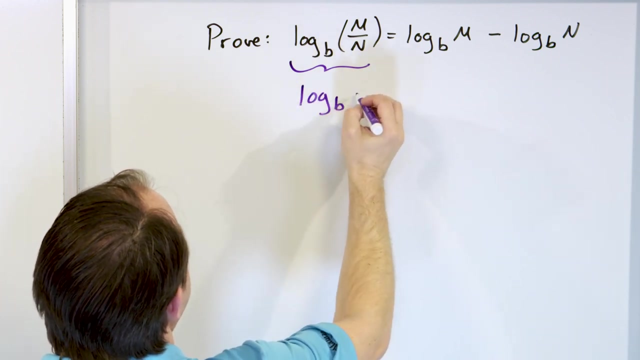 So, ultimately, this proof is going to be very, very similar to what we did before, But let me show you how we're going to get there. The first thing we're going to do is we're going to recognize that this statement right here is really the same as log base b of m multiplied by log base b of m. 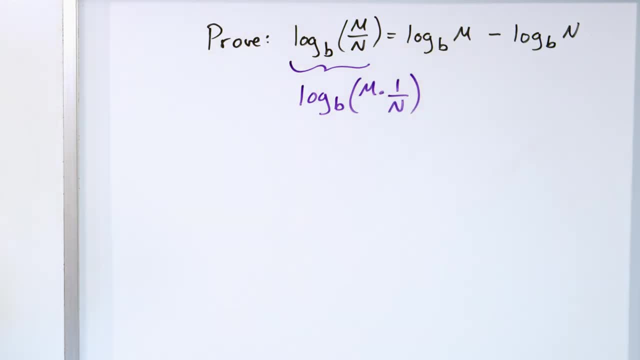 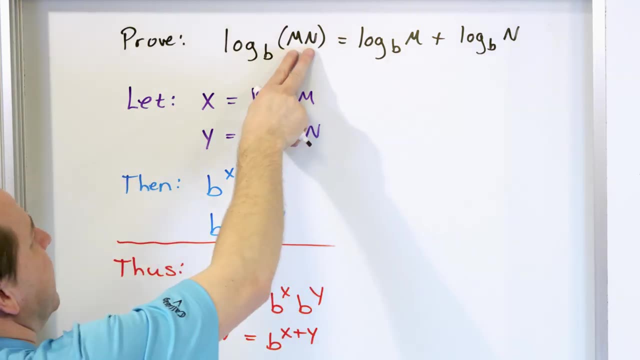 So we're going to multiply by 1 over n, right, Multiply by 1 over n. That's how you get a division here. You multiply by 1 over n, And since we know what happens when we multiply things, we can use a similar proof to go on. In fact, we could even use that thing, We could just. 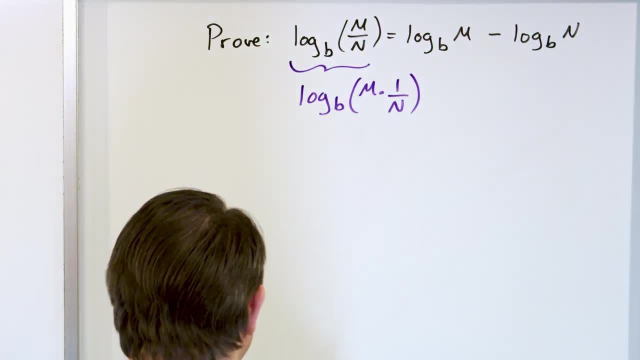 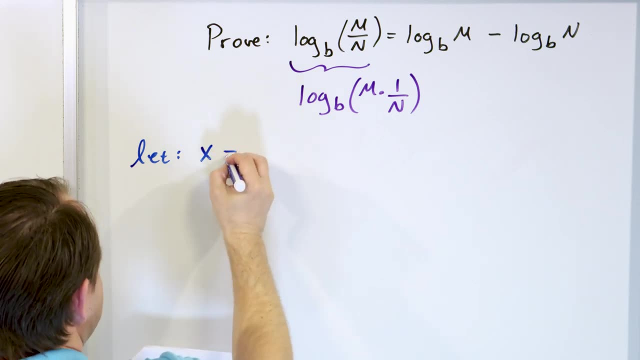 substitute in and use it, But that's no fun. Let's do it the real way. Let's do it the right way. Let's let the following things happen. Let's say: let's let x equal to the log base b of something. 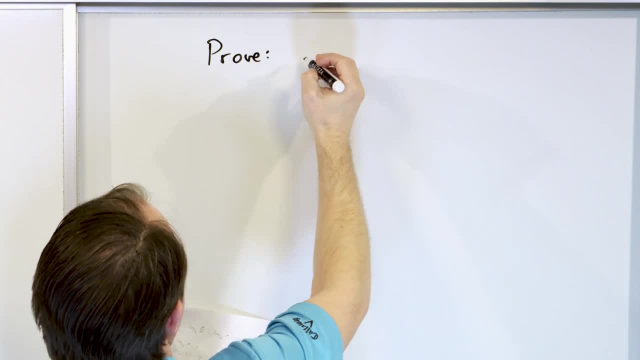 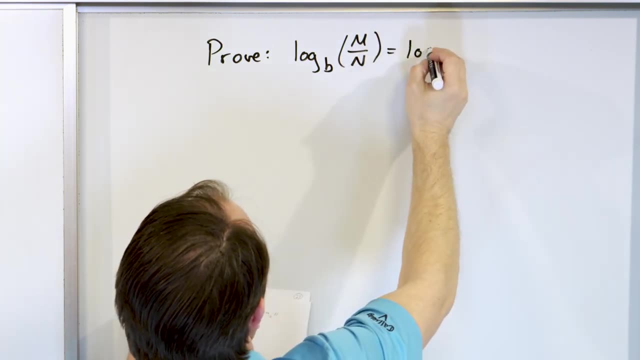 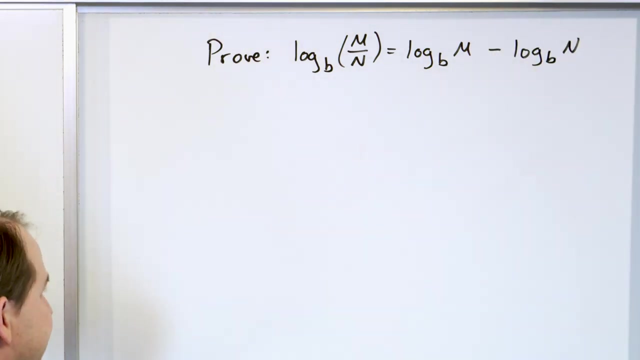 prove this last one. Prove the following thing: Log base b of the division m over n is equal to log base b of m minus sine log base b of n. So I want us to do the subtraction there. So So, ultimately, this proof is going. 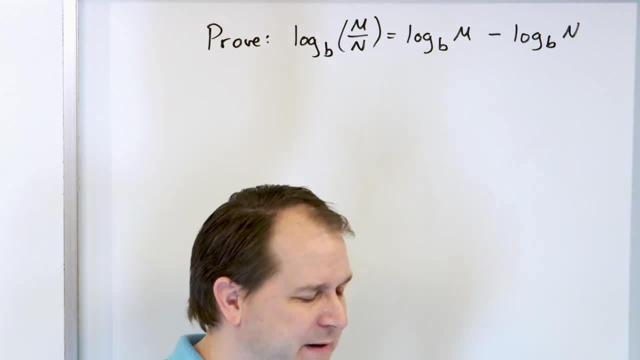 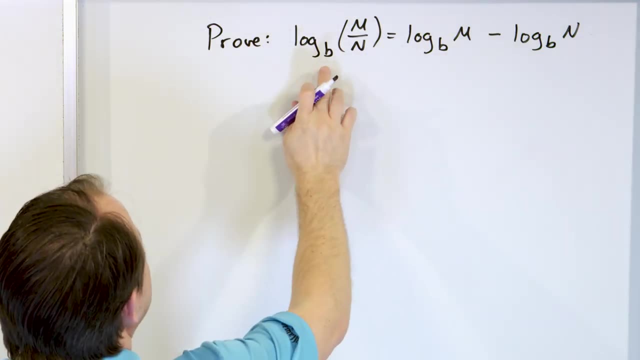 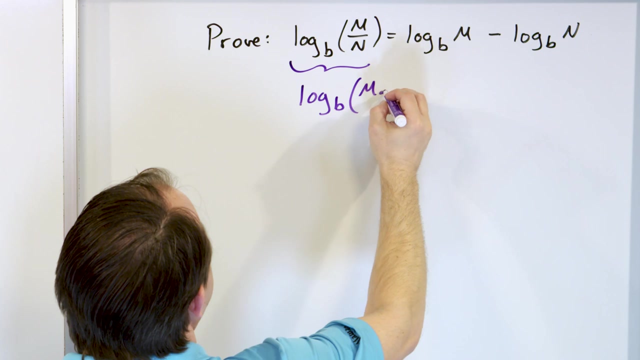 to be very, very similar to what we did before, But let me show you how we're going to get there. The first thing we're going to do is we're going to recognize that this statement right here is really the same as log base b of m multiplied by 1 over n. 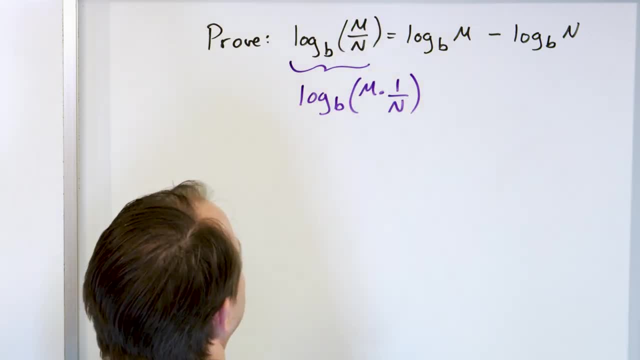 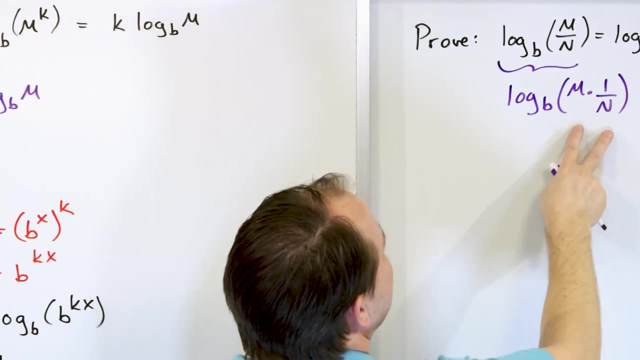 Multiply by 1 over n. That's how you get a division here. You multiply by 1 over n, And since we know what happens when we multiply things, we can use a similar proof to go on. In fact, we could even use that thing. 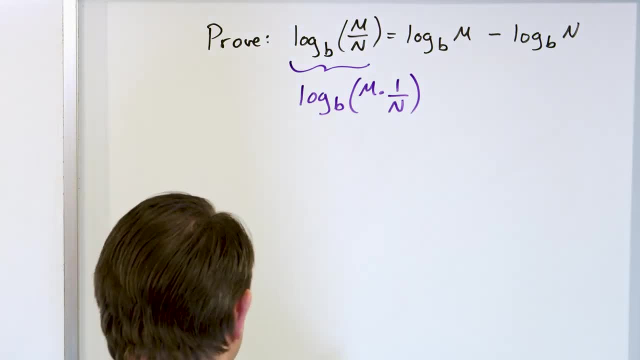 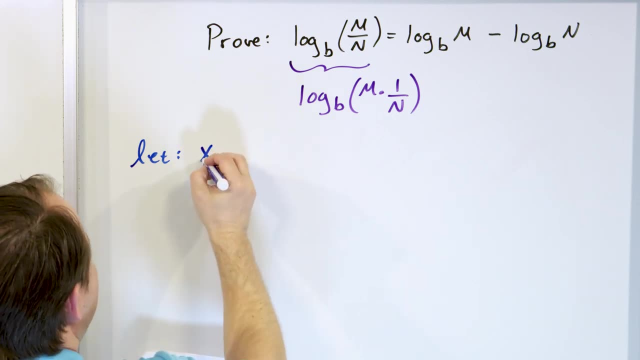 We could just substitute in and use it, But that's no fun. Let's do it the real way. Let's do it the right way. Let's let the following things happen: Let's let x equal to the log base b of something called m. 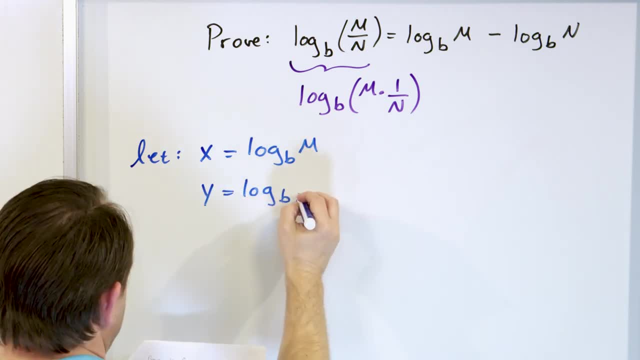 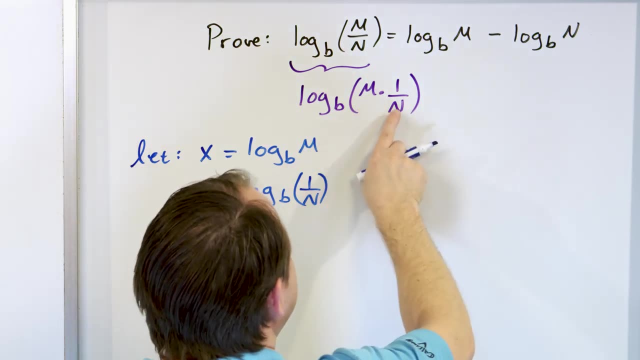 And we'll let y equal log base b of something called 1 over n, 1 over n, like this. Why am I doing that? Because I know I'm going to need an m and I know I'm going to need a 1 over n. 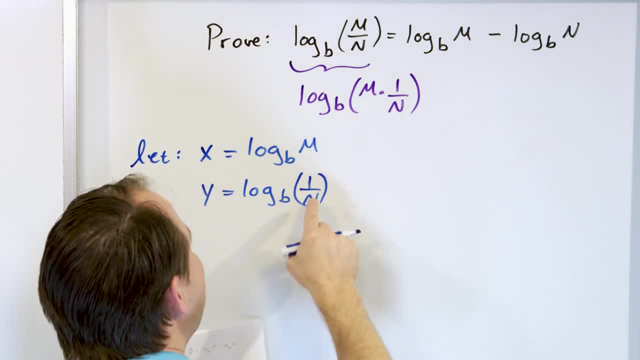 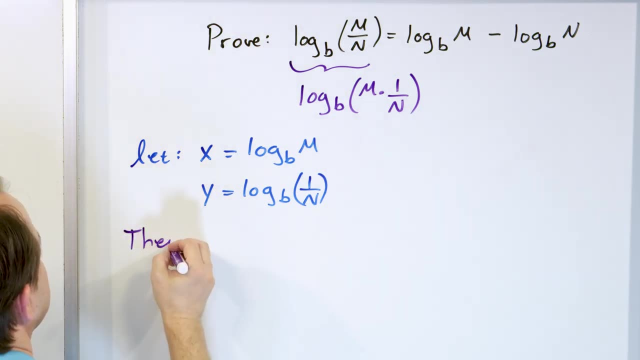 It's different than the other one, but even though we're just multiplied together, I'm going to need some fraction with an m on the bottom here, So we'll do the same thing again. Then the following things are true: b to the power of x is m. 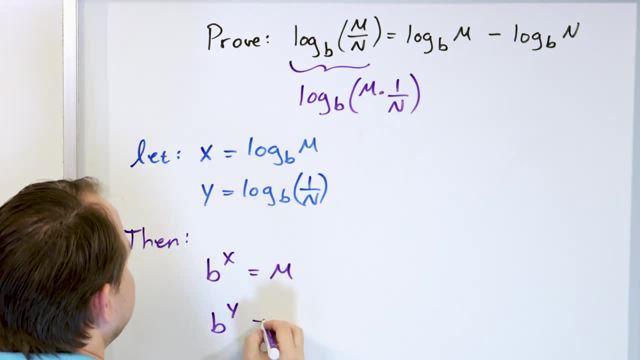 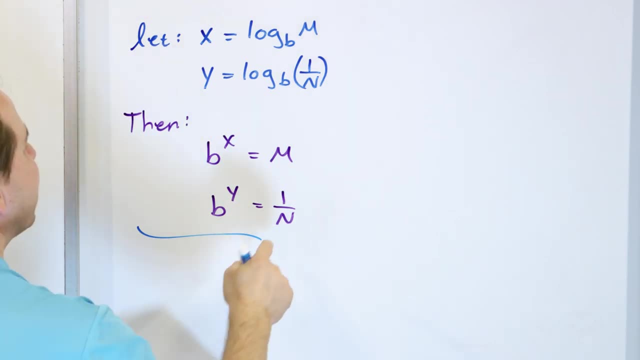 And then from this one b to the power of y is 1 over n, So we're going to need those All right Now, ultimately, what I'm trying to do is I'm trying to form the product of these things so I can take the logarithm right. 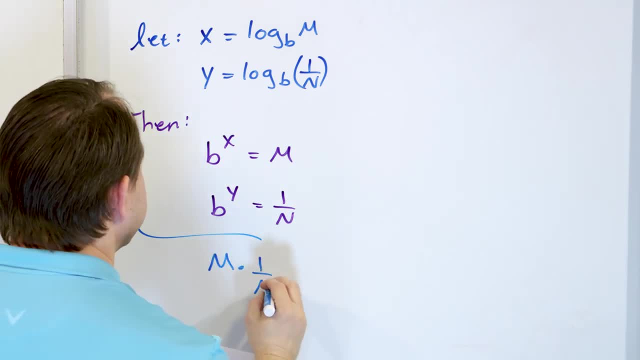 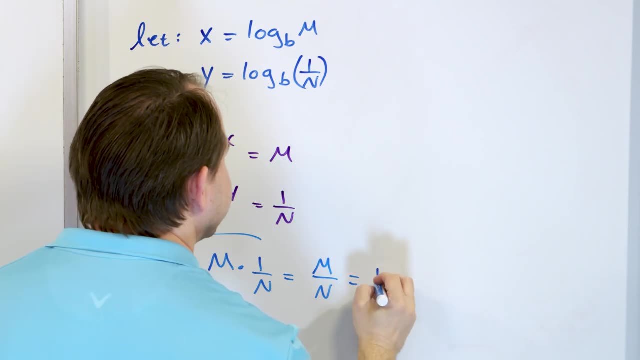 So what I'm going to have is m times 1 over n, because I'm trying to make m over n, is m over n, But I know what these things are equal to: It's b to the x times b to the y, because that's m. 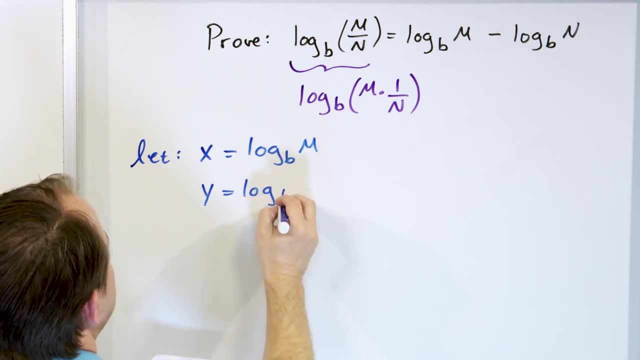 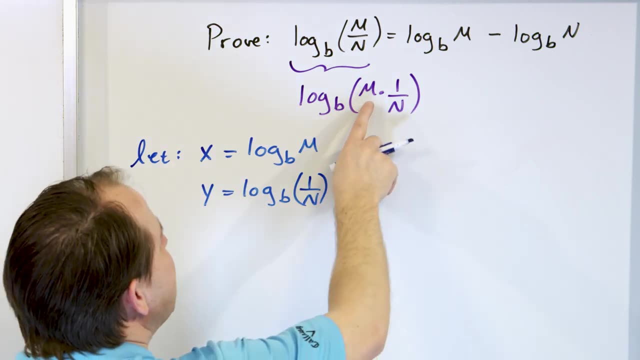 called m And we'll let y equal log base b of something called 1 over n, 1 over n like this. Why am I doing that? Because I know I'm going to need an m and I know I'm going to need a 1 over n. It's. 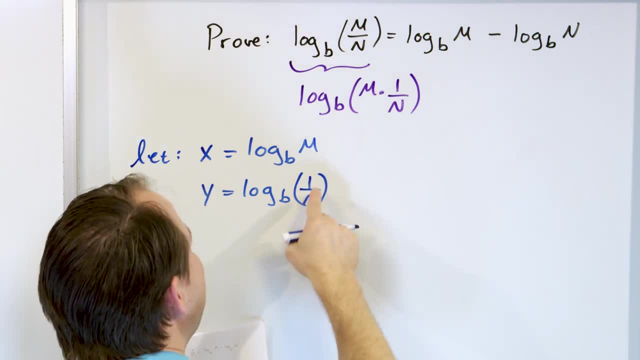 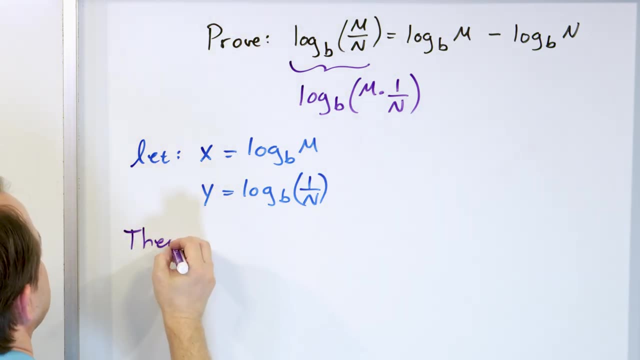 different than the other one. They were just multiplied together. I'm going to need some fraction with an m on the bottom here. OK, So we'll do the same thing again. Then the following things are true: b to the power of x is m, And then from this one: 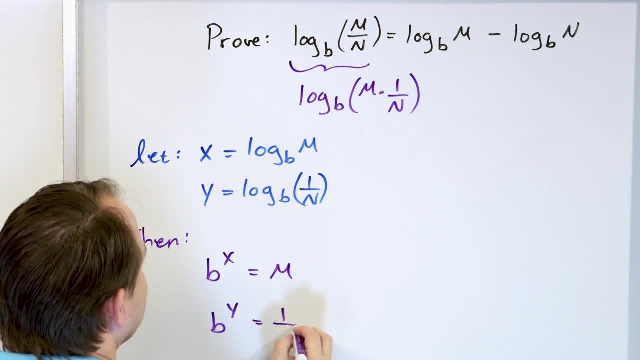 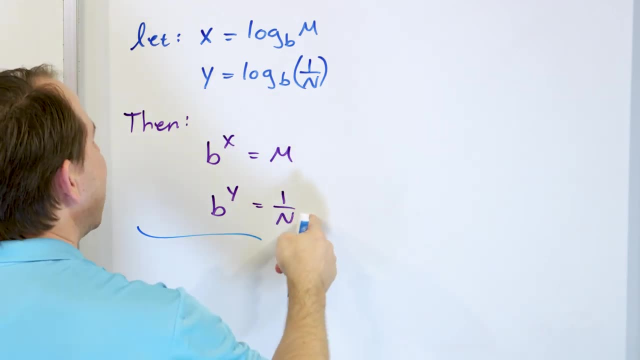 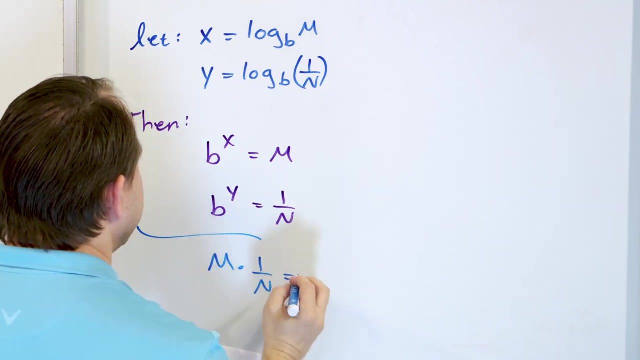 b to the power of y is 1 over n, So we're going to need those All right Now. ultimately, what I'm trying to do is I'm trying to form the product of these things so I can take the logarithm right. So what I'm going to have is m times 1 over n, because I'm 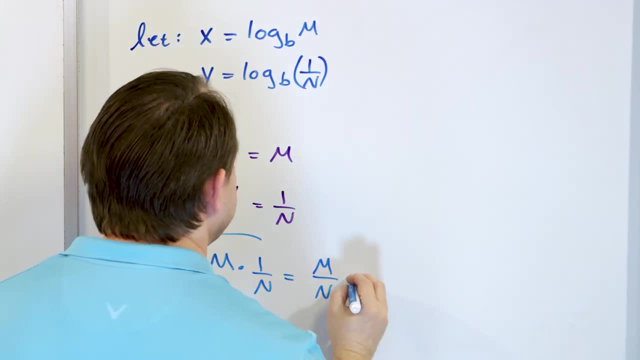 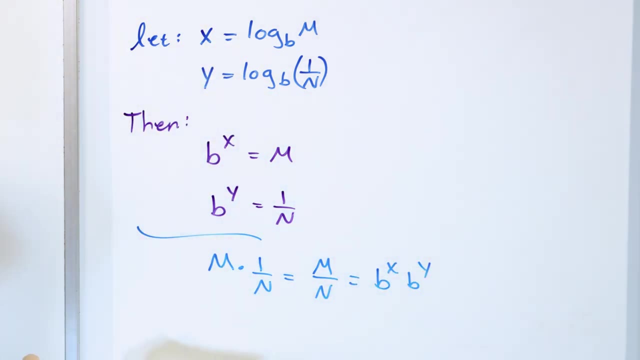 trying to make m over n is m over n. But I know what these things are equal to. It's b to the x times b to the y, because that's m and that's 1 over n. OK, But what is this? b to the x plus y? So what I figured out is m over n is exactly the same thing. 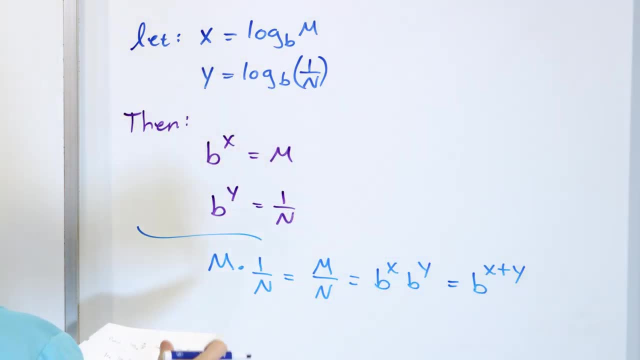 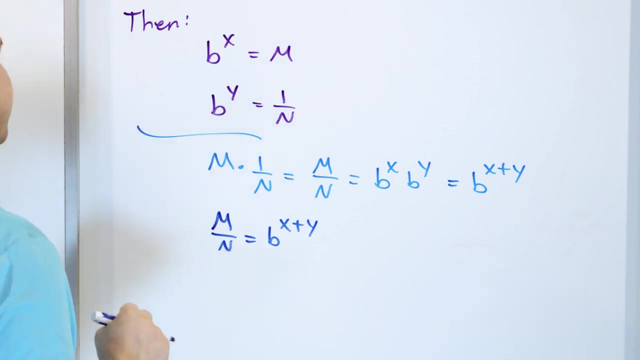 as b to the x plus y. So I'm going to take and write that down separately: m over n is b to the x plus y. And now I want to take the logarithm of both sides. Why? Because I want the logarithm. 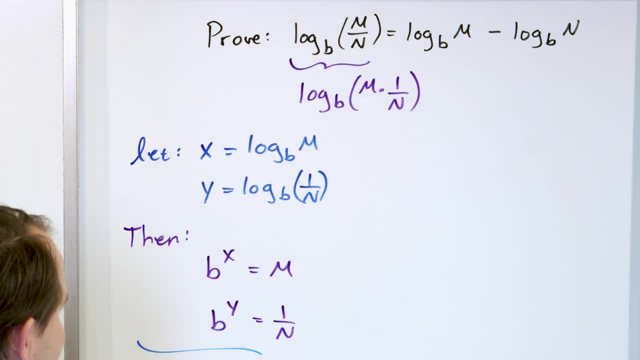 of this quotient, of this division. That's what I'm trying to get to. I'm trying to take the logarithm of that. So I had to kind of do all of this to get to where I had an expression for this, And so I'll take the logarithm of this quotient and I'm trying to get to the logarithm of. 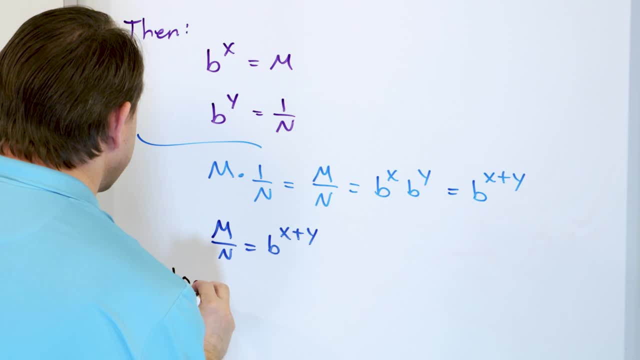 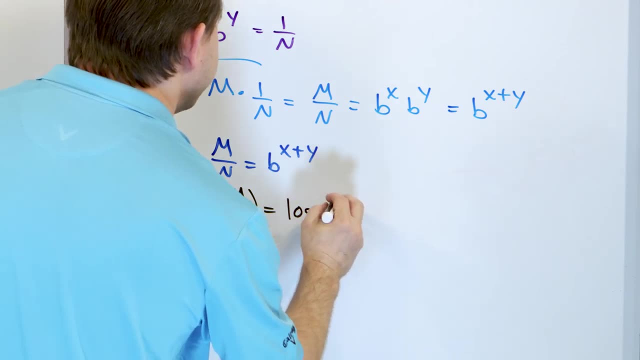 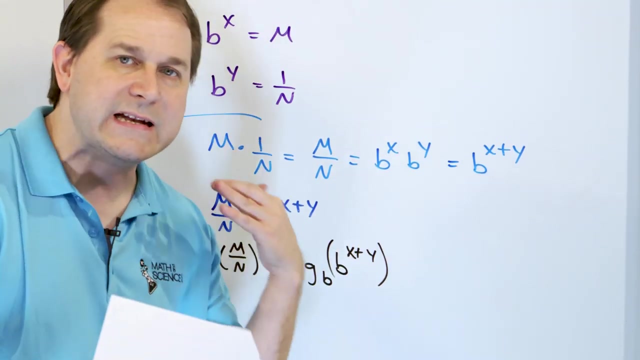 the logarithm of both sides, So it has to be a base b logarithm. Base b of m over n equals log base b of b to the x plus y. All of this is wrapped up inside that logarithm. Now I have the same thing happening on the right, The logarithm of an exponential annihilate each. 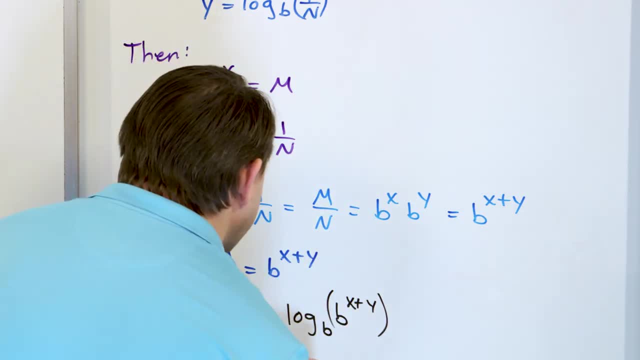 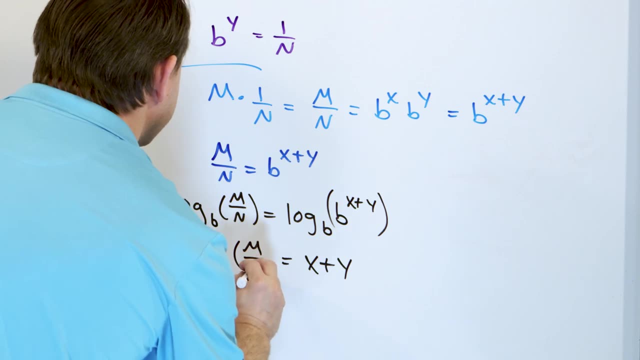 other. All I'm going to have on the right-hand side is x plus y. On the left-hand side I'll have log base b m over n like this. All right, so what am I going to have next? I know what: x and. 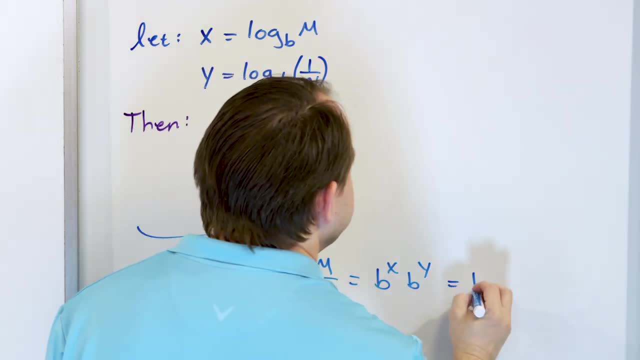 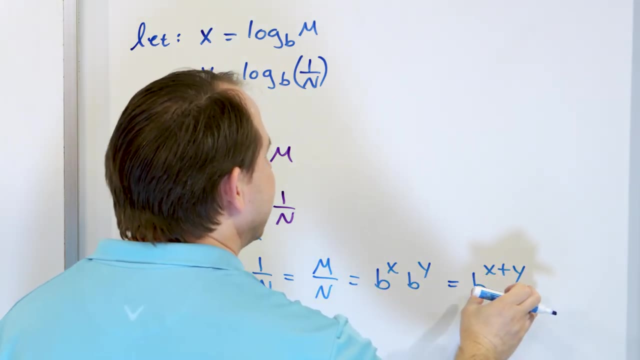 and that's 1 over n. OK, But what is this? b to the x plus y. So what I figured out is m over n is exactly the same thing as b to the x plus y. So I'm going to take and write that down separately. 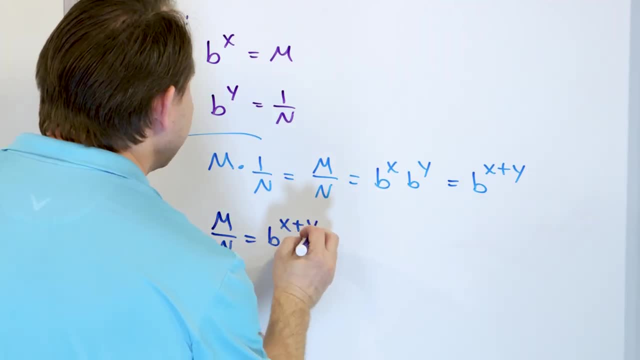 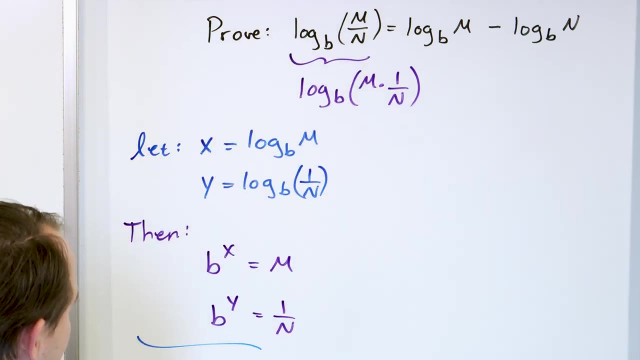 m over n is b to the x plus y, And now I want to take the logarithm of both sides. Why? Because I want the logarithm of this quotient, of this division. That's what I'm trying to get to. I'm trying to take the logarithm of that. 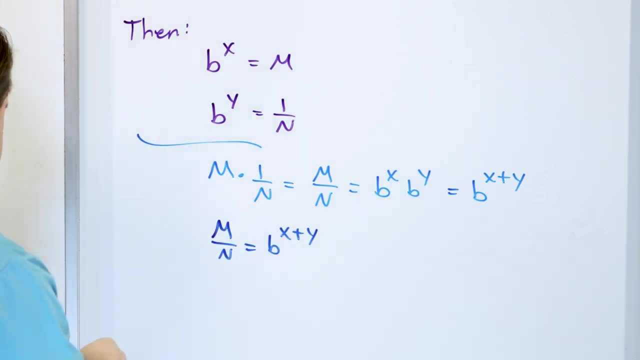 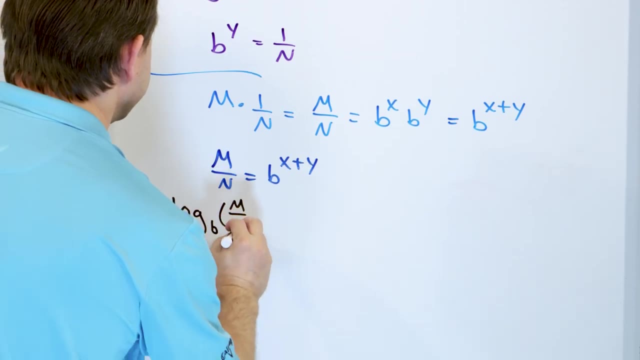 So I had to kind of do all of this to get to where I had an expression for this, And so I'll take the logarithm of both sides. So it has to be a base b- logarithm. base b of m over n. 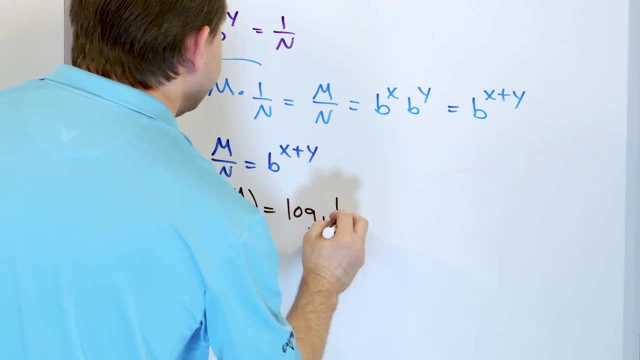 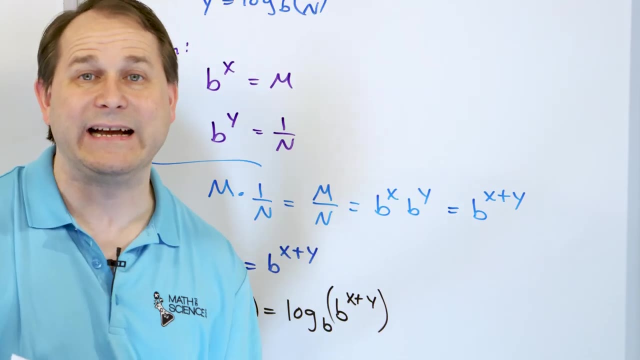 That's going to be. m over n equals log base b of b to the x plus y. All of this is wrapped up inside that logarithm, And I have the same thing happening on the right, The logarithm of an exponential annihilate each other. 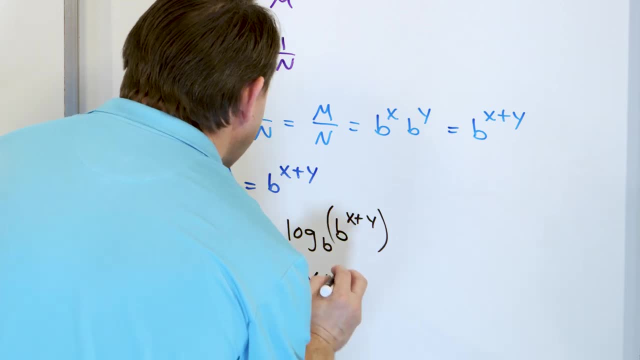 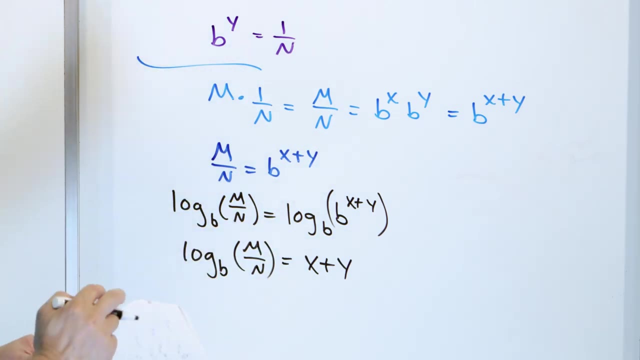 All I'm going to have on the right-hand side is x plus y. On the left-hand side, I'll have log base b m over n like this. All right, So what am I going to have next? I know what x and y are. 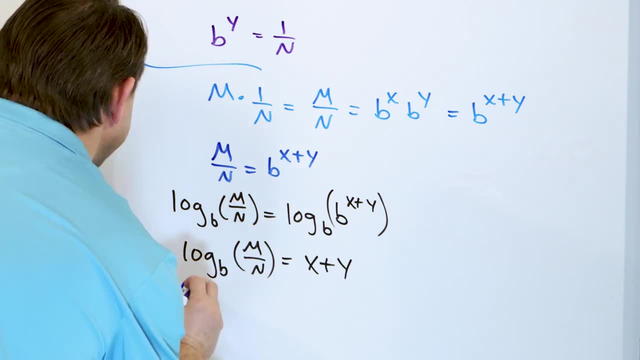 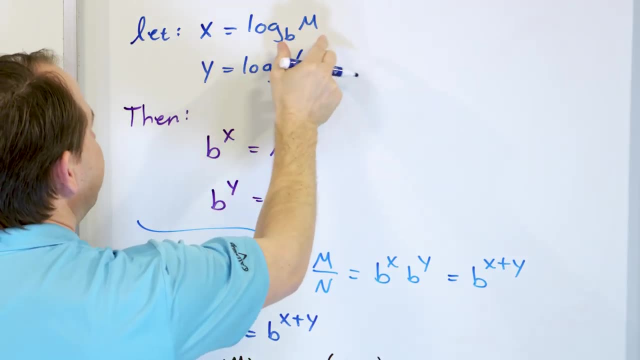 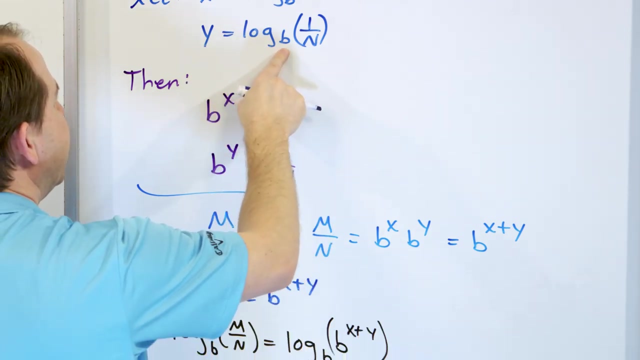 I know that log base b m over n is equal to x plus y, But I know what x and y are. x is base b log of m. log base b of m. And then the y is this guy: log base b 1 over n. 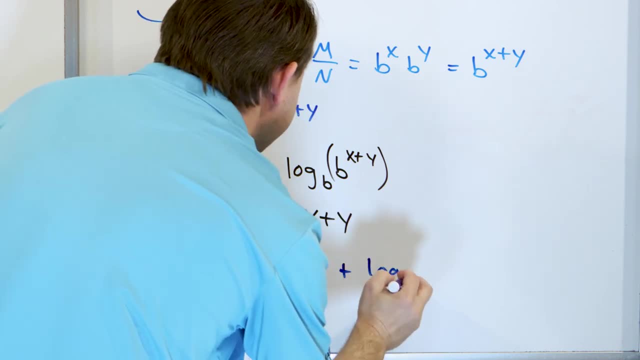 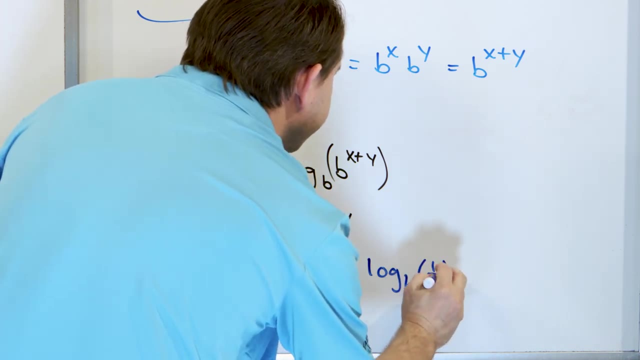 So it's plus sign from this log base: b 1 over n. It's hard to read. I'm sorry about that. This is a capital N right here, Like this: So x plus y. So I'm just plugging what I have. 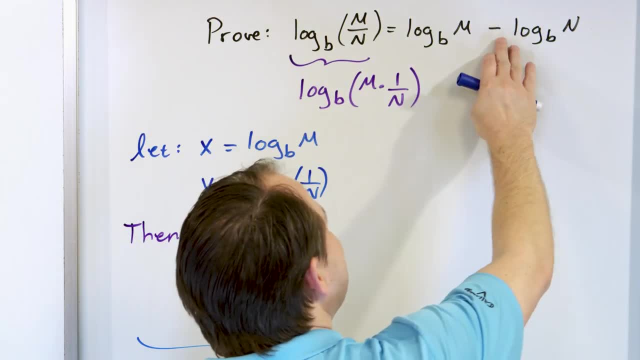 Now you think, well, this isn't quite right, This is a plus sign, This is a minus sign. It's not quite right, But we're going to get there. How are we going to get there? Let's go, hmm. 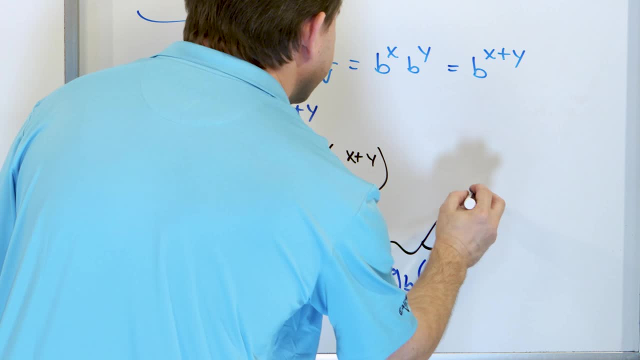 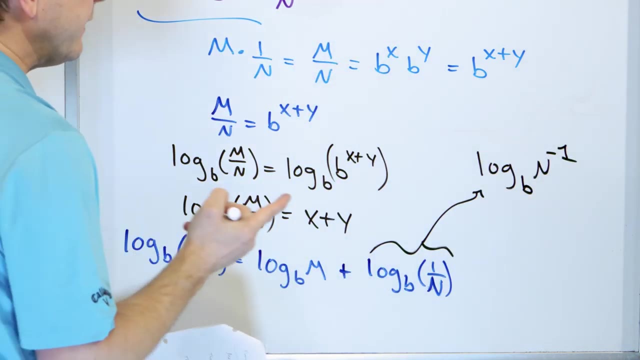 Well, if you think about it, let me go over here. Let me just write a note over here. This is the same thing as the logarithm base b of n to the minus 1.. How do I know that? Because 1 over n is the same thing as n to the minus 1.. 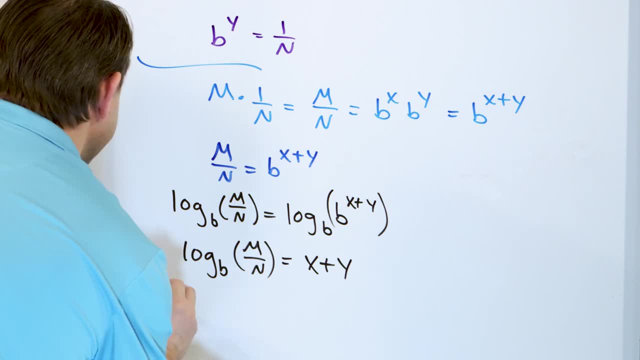 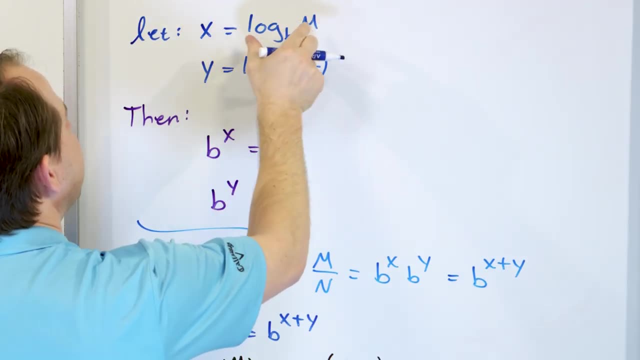 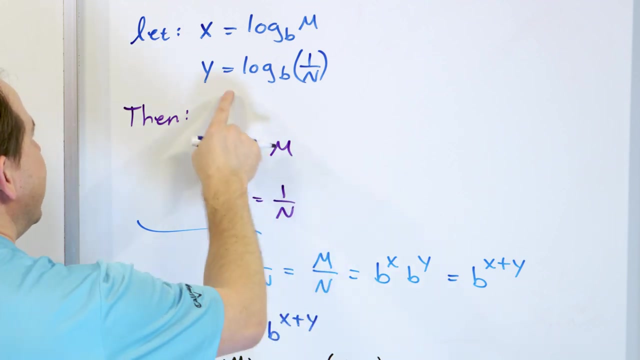 y are. so let's substitute for that Log base b. m over n is equal to x plus y. but I know what x and y are. x is log base b. log of m. log base b of m. and then the y is this guy log base b. 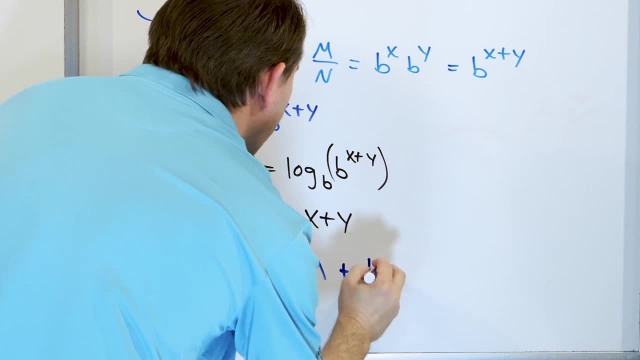 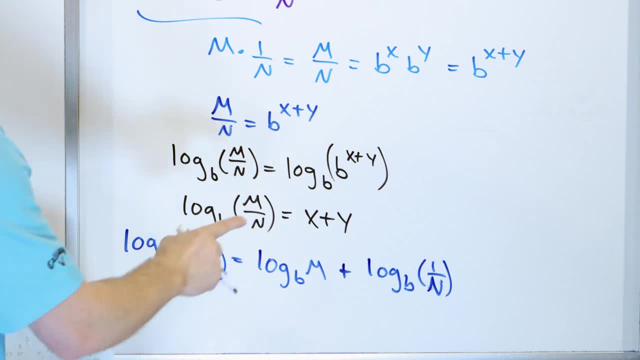 that This is a capital N right here, like this: So x plus y. So I'm just plugging what I have. Now you think, well, this isn't quite right. This is a plus sign, This is a minus sign. It's not. 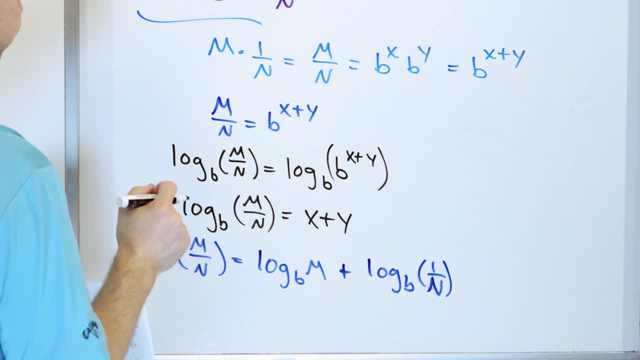 quite right, but we're going to get there. How are we going to get there? Let's go. well, if you think about it, let me go over here. Let me just write a note over here. This is the same thing as. 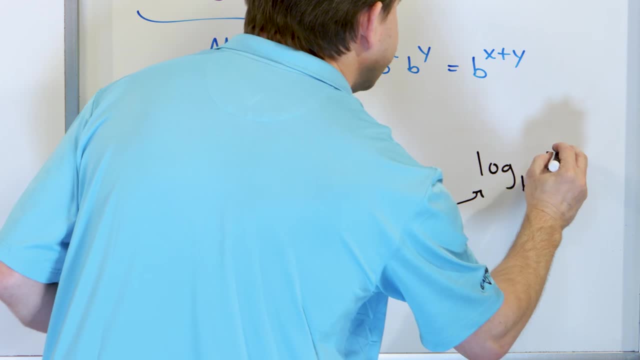 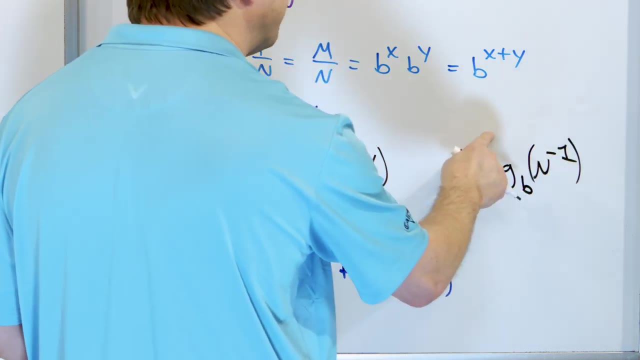 the logarithm Base b of n to the minus 1.. How do I know that? Because 1 over n is the same thing as n to the minus 1.. So this is an exponent, So this exponent can come out in front here. So then I have log. 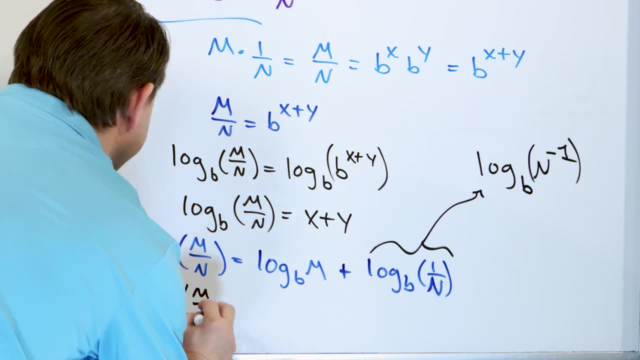 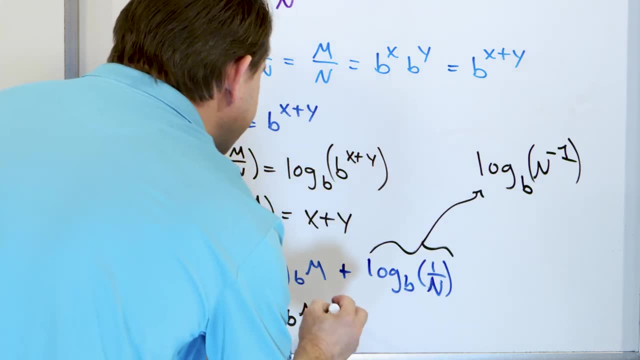 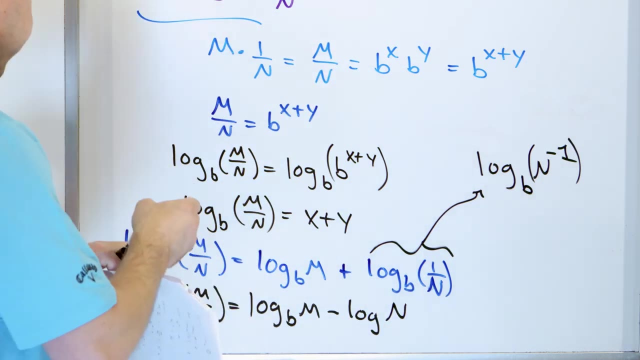 base b of m over n equals log base b of m And because of this the exponent could come down. It's going to be a minus sign log and then you have an n right here, And this is exactly what we're trying to prove. The log of the division of n, m divided by n, is the log of m minus the log. 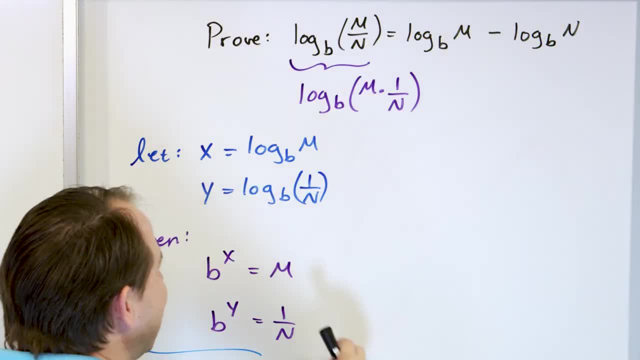 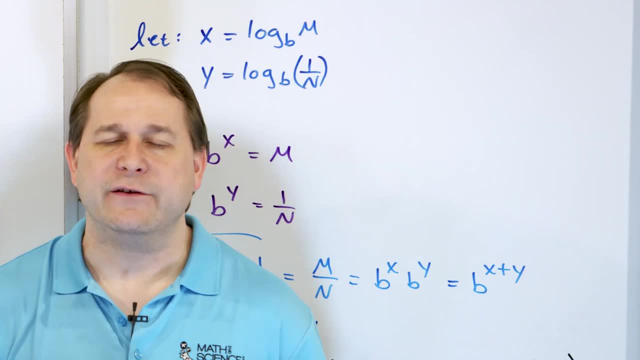 of n. It's exactly what we have right here. It all comes from this little exponent and it comes from having to define things this way. so I can make the product of m and n So or the division of m divided by n. Do I expect you to know this? No, of course. not The first time you see this- nobody. 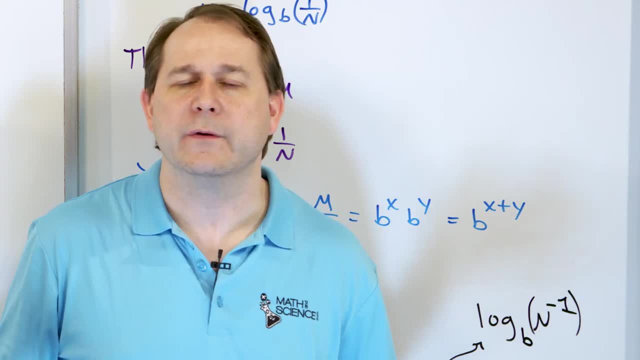 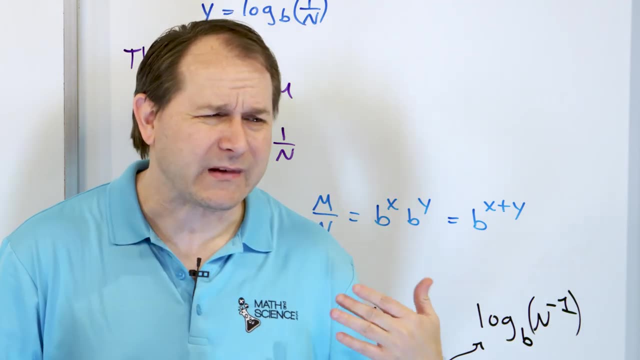 knows how to do this stuff. All I care about is that you can follow through. So it serves two purposes. It sharpens your skills so that you know where things come from. I mean, you know how to use these laws of logarithms in order to make logical conclusions. 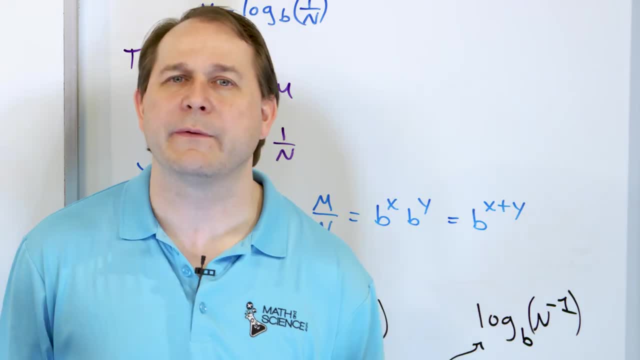 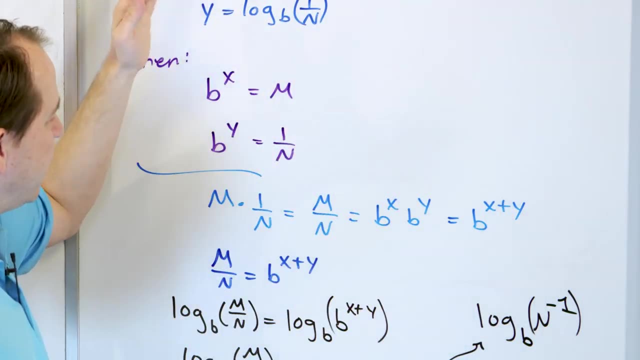 And it also shows you that these laws of logarithms don't just come from the sky. They come from logical progression of thought. We start from here. We let this equal to this Notice how nobody- I don't want to say nobody- on this earth. There's some pretty brilliant math guys out there, But not. 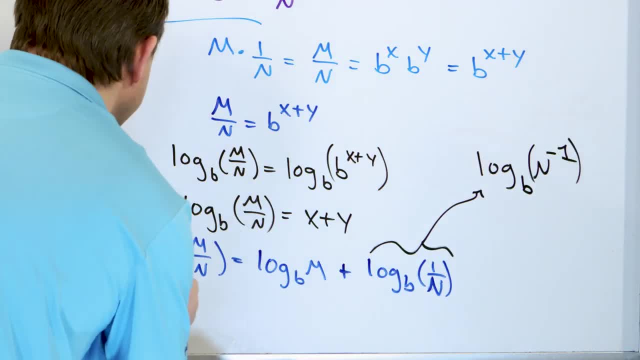 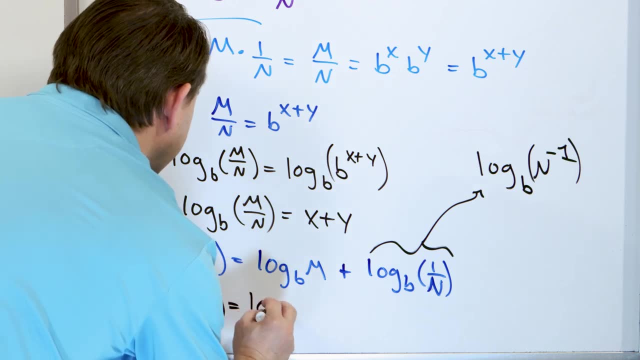 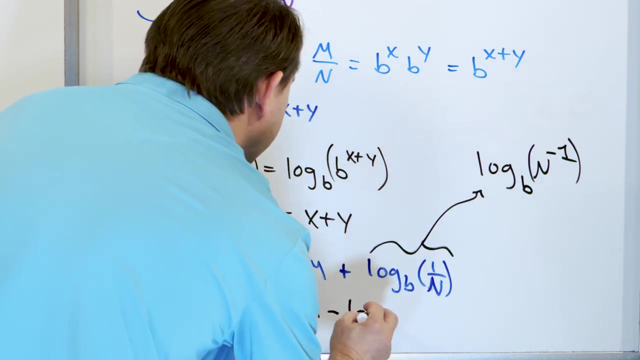 So this is an exponent, So this exponent can come out in front here Here. And then I have log base b of m over n equals log base b of m And because of this the exponent could come down. It's going to be a minus sign log. 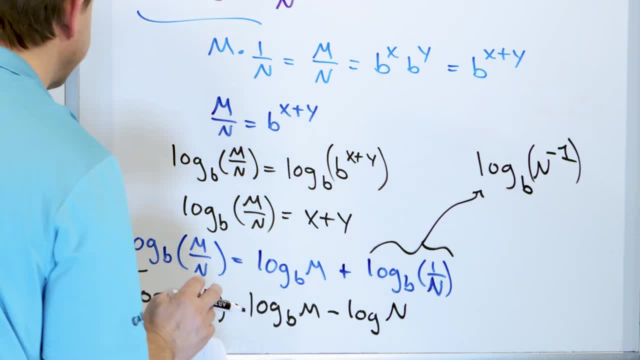 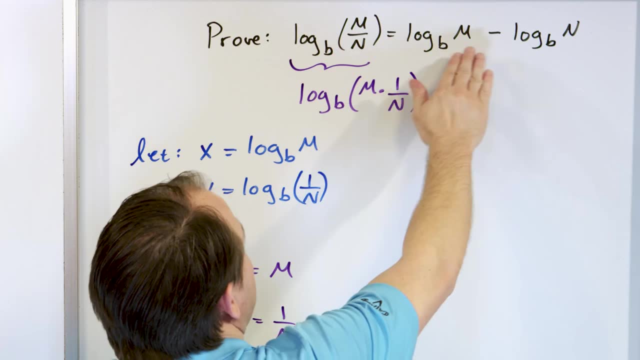 And then you have an n right here, And this is exactly what we're trying to prove. The log of the division of n, m divided by n, is the log of m minus the log of n. It's exactly what we have right here. 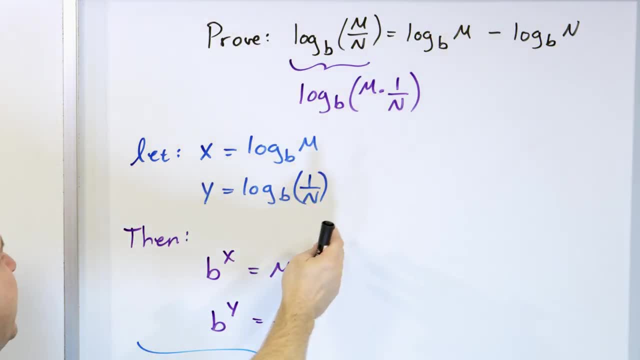 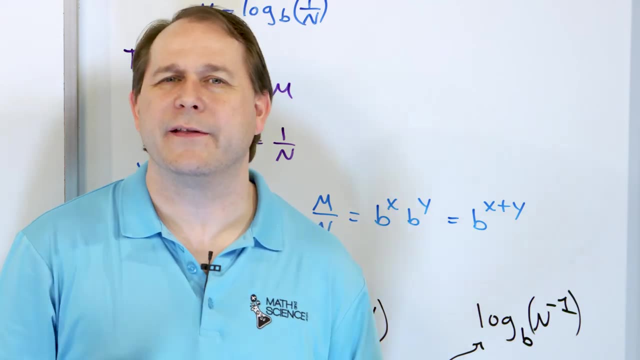 It all comes from this little exponent And it comes from having to define things this way, So I can Make the product of m and n, Or the division of m divided by n. Do I expect you to know this? No, of course not. 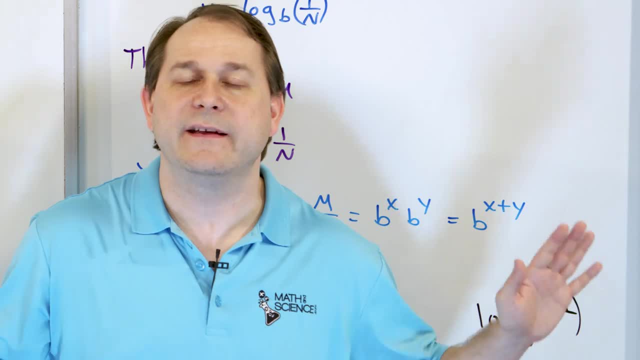 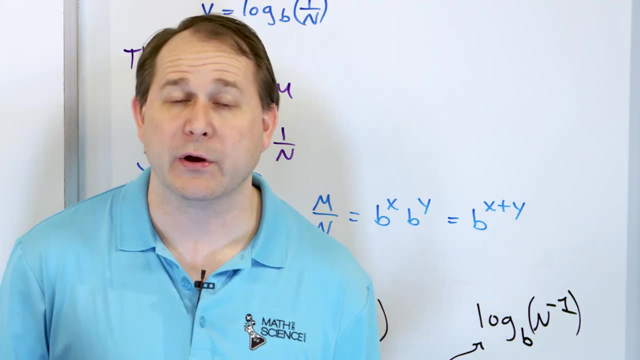 The first time you see this. nobody knows how to do this stuff. All I care about is that you can follow through. So it serves two purposes: It sharpens your skills so that you know where things come from. I mean, you know how to use these laws of logarithms. 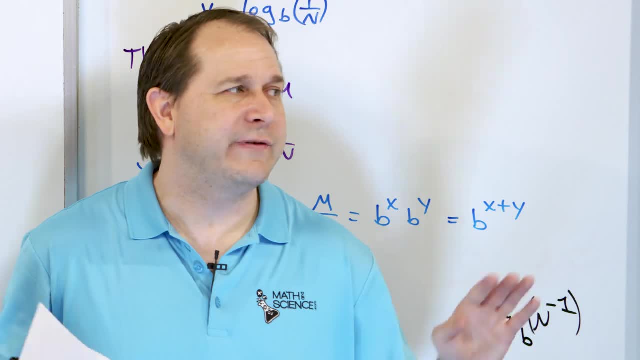 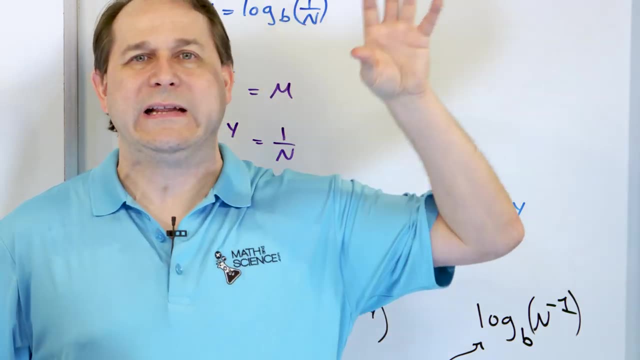 in order to make logical conclusions. And it also shows you that these laws of logarithms don't just come from the sky. They come from logical progression of thought. We start from here. We let this equal to this. Notice how nobody- I don't want to say nobody- on this earth. 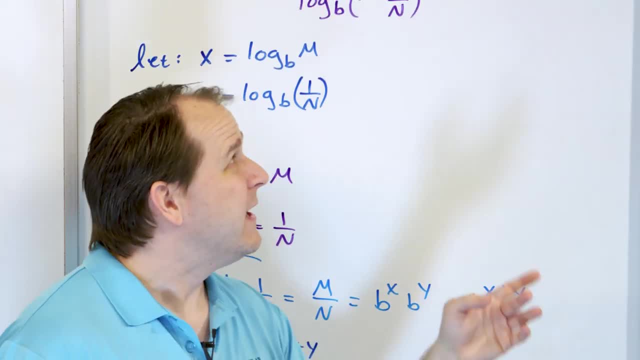 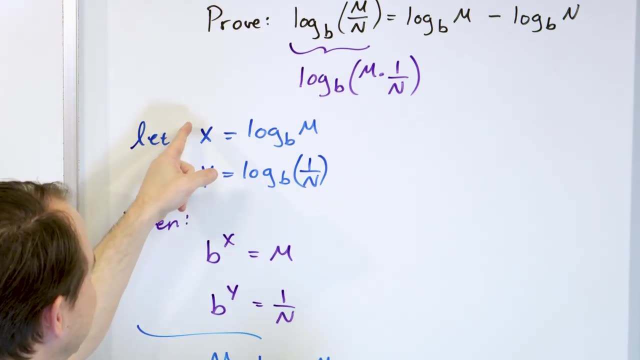 There's some pretty brilliant math guys out there, But not very many people can look at this and say: oh yeah, I know how to prove that, No problem, I can see all the steps. Almost nobody can do that, But what we can say is: if we let this, equal to this. 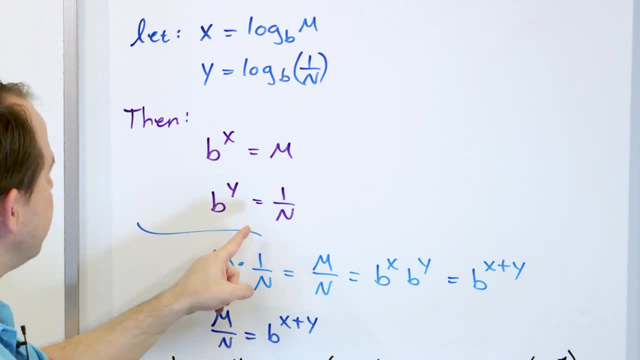 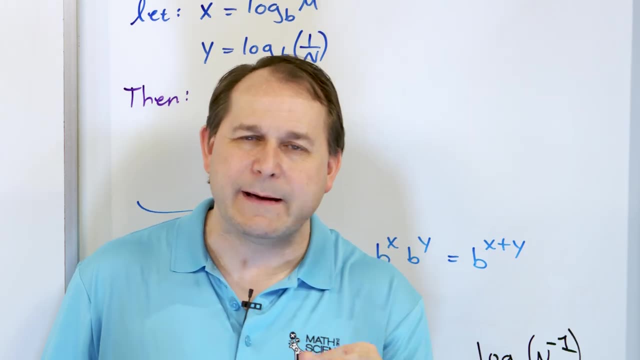 and this equal to this, then this must be true. Then, if we multiply this and this, it must be this times this, And then we just ripple through. Every little step is an incremental step towards the finish line. That's all I care, that you understand. 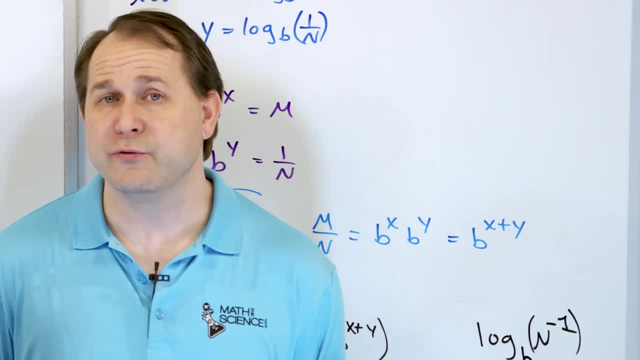 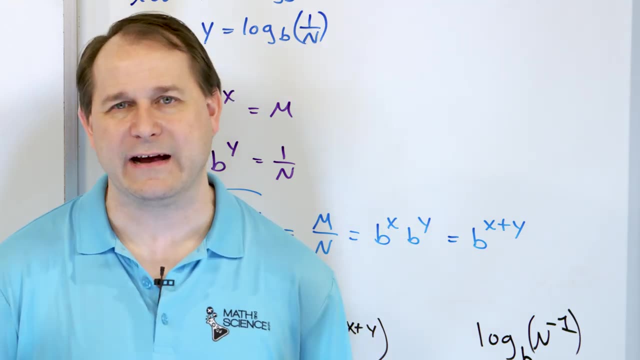 So make sure you understand this. If you want to grab a sheet of paper and prove these yourself, It definitely can't hurt you. And then follow me on to the next lesson. We're going to start to learn more about the applications of logarithms and exponentials. in math. 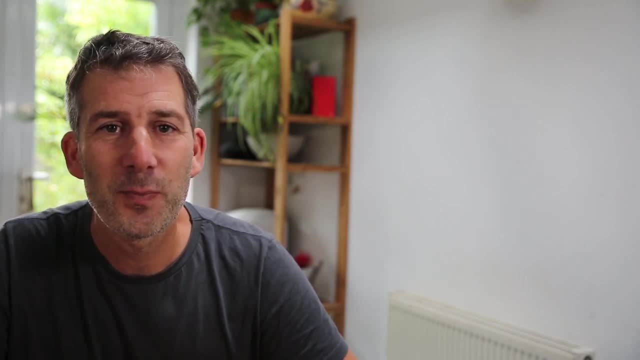 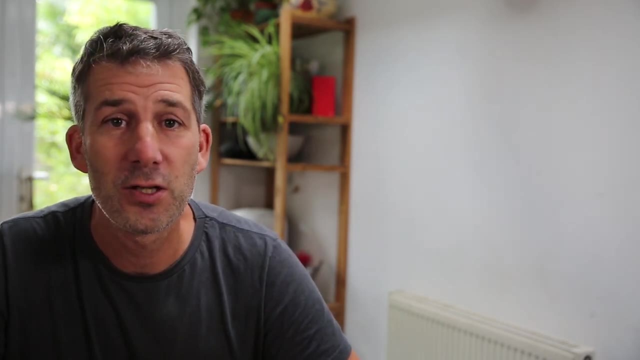 Hello, today we're looking at mental and written methods for finding percentages of an amount. So what I mean by that is that we're going to be able to do things like to find 15% of 82, but without using a calculator. I'm going to be using these.